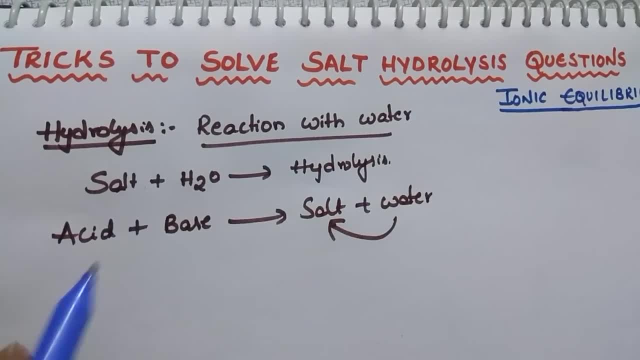 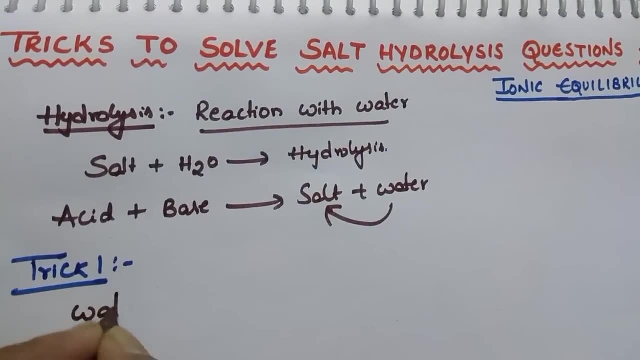 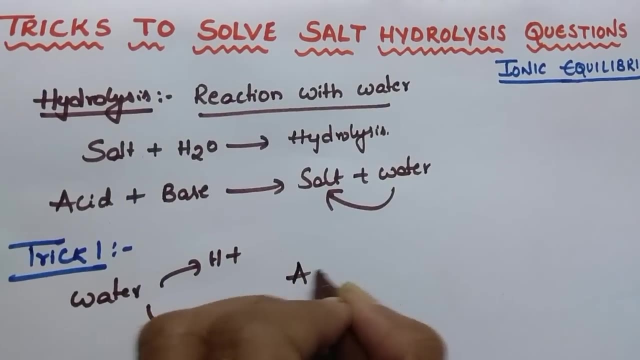 reaction will take place. Let us see the trick number one: How water dissociates Students. water dissociates into H plus and OH minus. I am taking the salt AB. Suppose it dissociates into A plus and B minus, Then what happens? 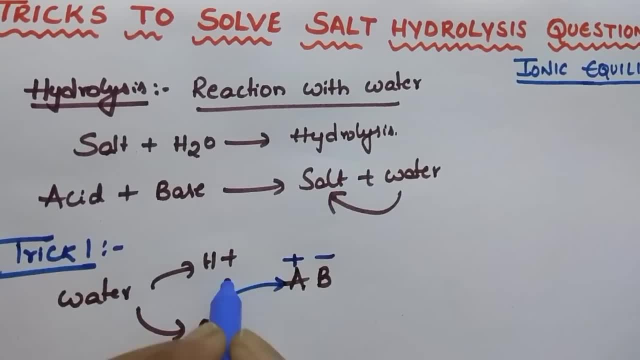 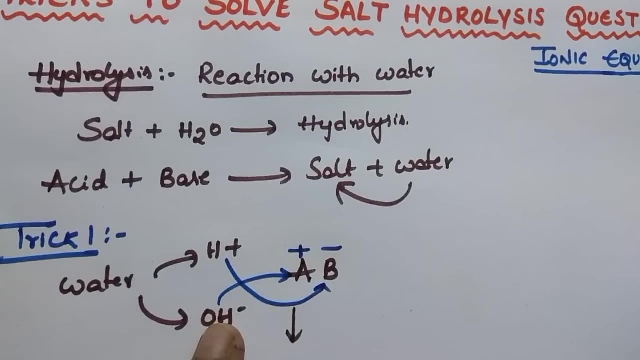 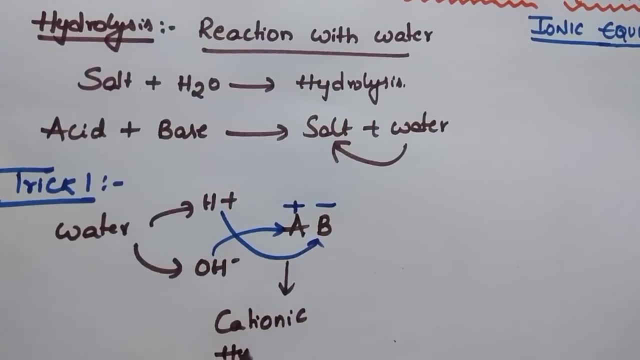 This A plus reacts with this OH minus. Then this H plus attacks this B minus. What happens here? This A plus is reacting with OH part of water, and this is called as cationic hydrolysis. Why? Because here cation is undergoing the reaction. That's why it is called as cationic hydrolysis. 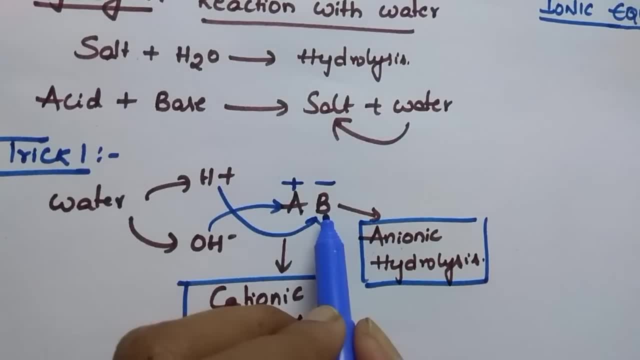 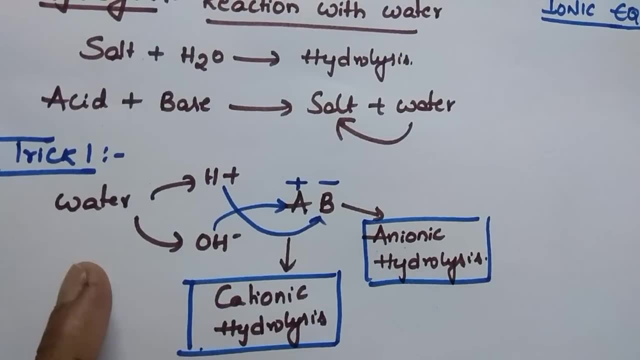 In the same way, anion of the salt reacts with the H plus of the water, Just opposite charges, you see, students. Then it forms a salt, It forms the compound which we call it as this process, We call it as anionic hydrolysis, because here anion is. 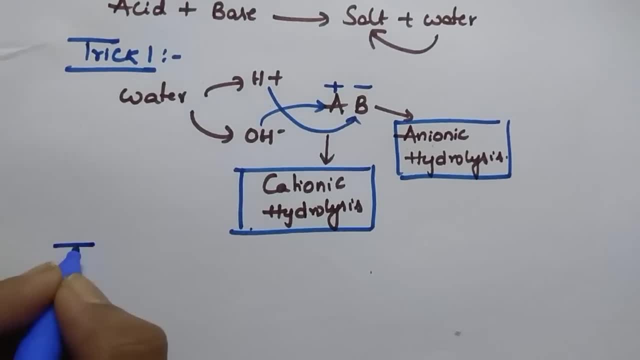 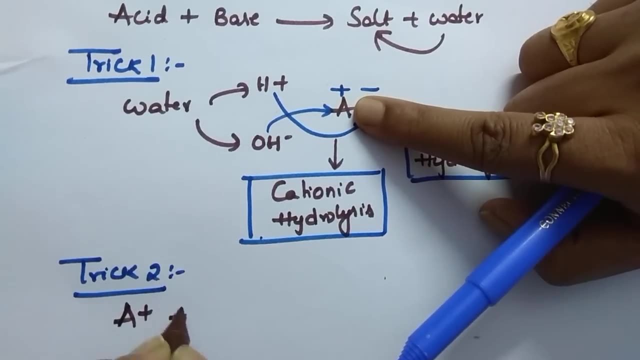 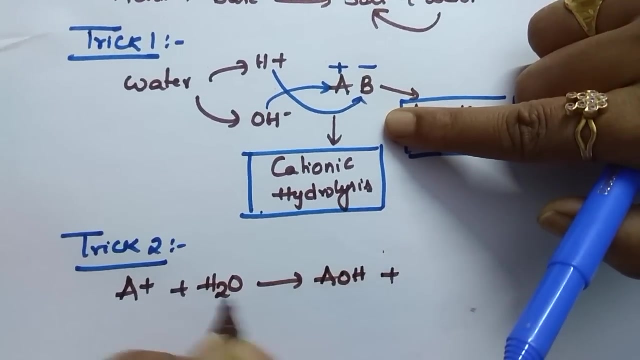 reacting. This is most important. Let us see trick number two. Until what I am telling you here, This is a cation A plus which is reacting with water. In water it reacts with the OH minus part and it forms AOH and it releases. 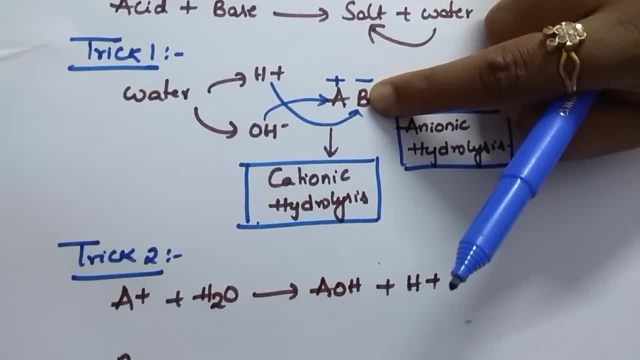 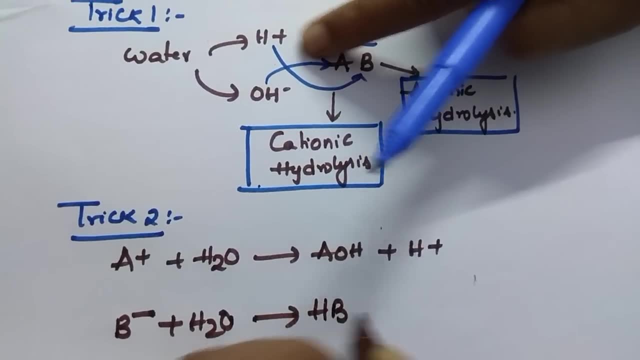 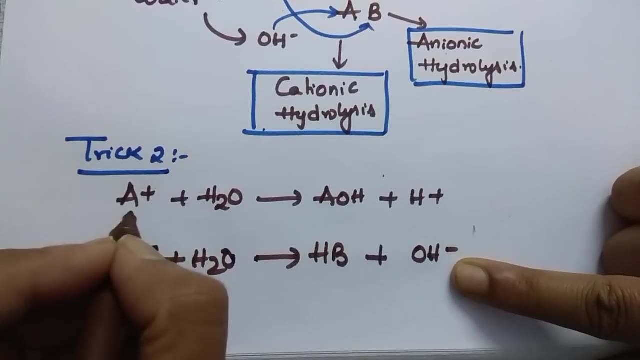 vicious H plus. and in the same way, this B is reacting with h plus of water. and what it forms? it forms hb. and which is it releases? it releases oh minus. just it takes h plus and it gives oh minus. what i want to say is: cation gives. 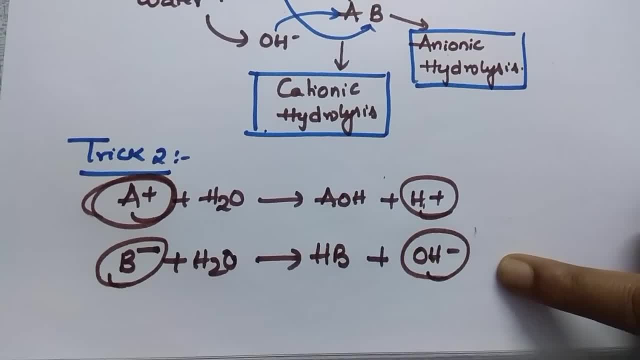 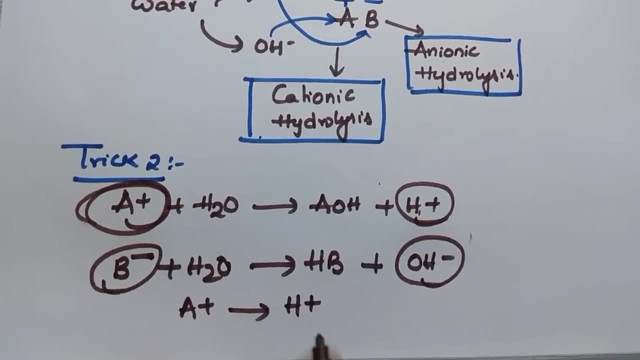 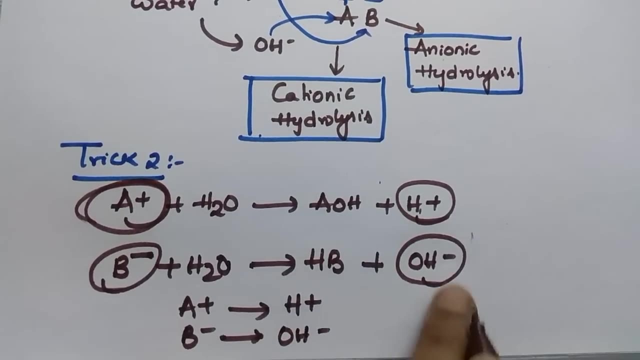 cation anion gives anion most. most important. where students get confused here: cation during cationic hydrolysis: first you have to calculate h plus and concentration during anionic hydrolysis: first you have to calculate oh minus ion concentration. if here you calculate directly, 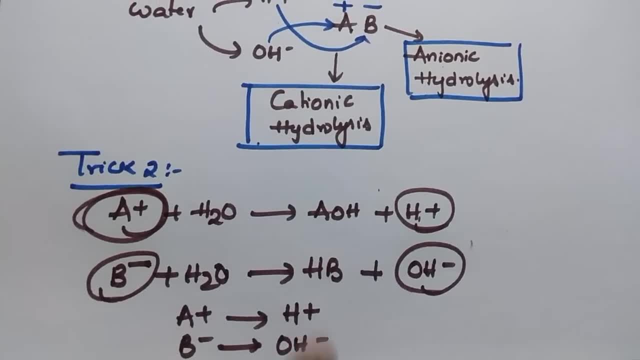 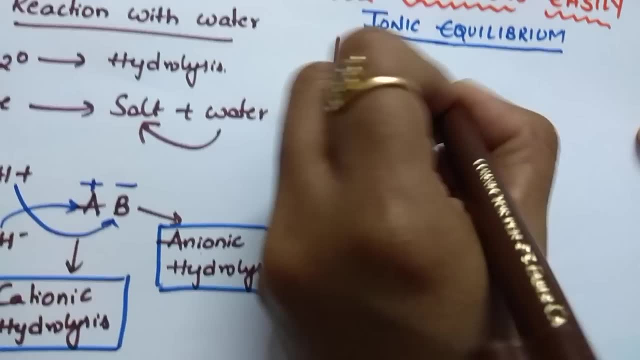 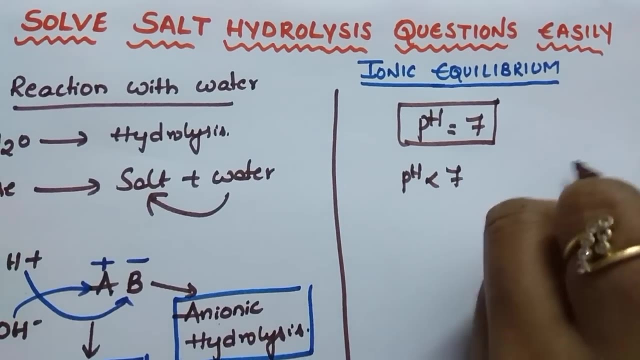 h plus, then your answer going to be wrong. i'll tell you how. don't worry of this. and one more thing is: generally ph is equal to 7 for neutral solutions. when ph is less than 7, then the solution is acidic and ph is greater than 7. the solution is basic here. if you get h plus ion concentration, 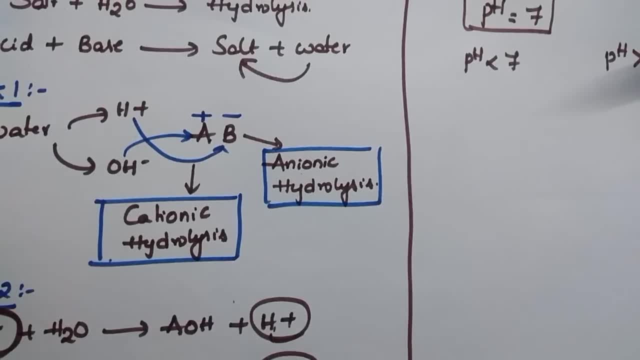 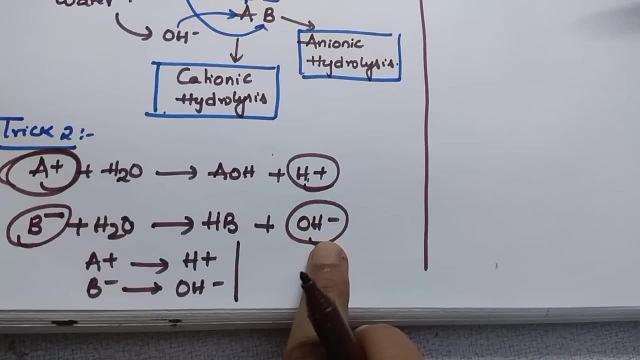 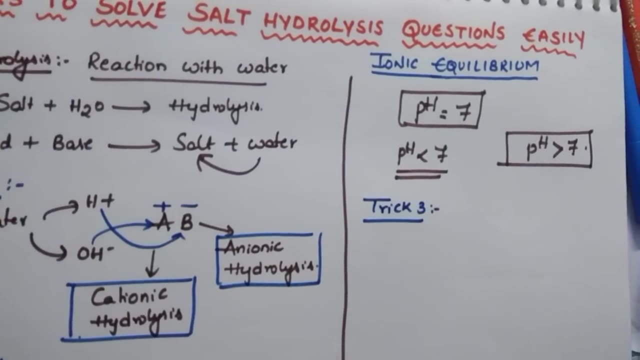 during cation anionic hydrolysis, then ph will be less than 7. and here what happens is during anionic hydrolysis, oh minus ion concentration is released and the ph will be greater than 7. trick number 3 student should be able to identify what kind of salt it is, suppose if you take nh4cl. 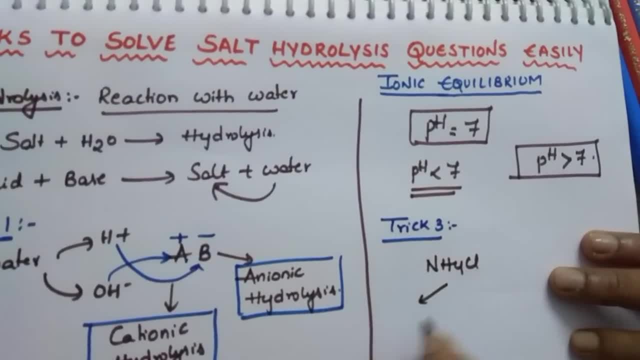 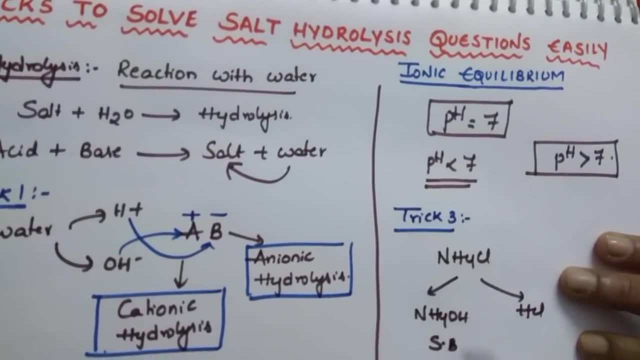 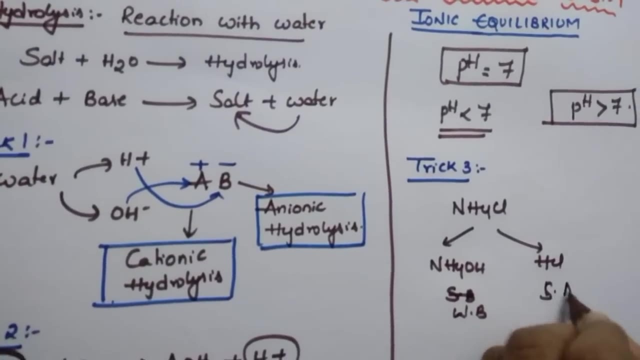 this one. it is a salt of weak base and strong acid. This is most important in salt hydrolysis. You have to identify that it is a salt of weak base and strong acid. If you don't know so, for example, if you take NaCl, NaCl is a salt of. 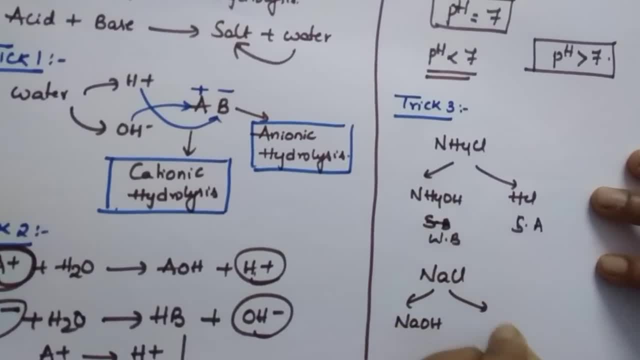 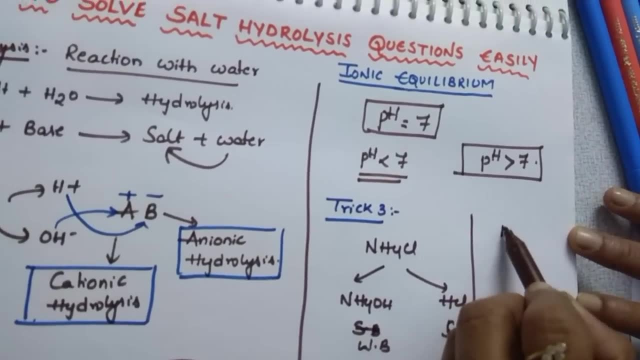 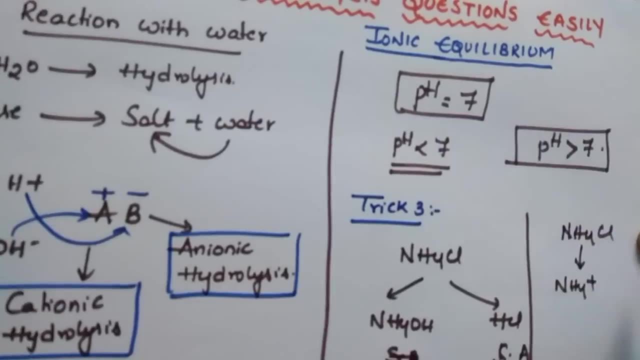 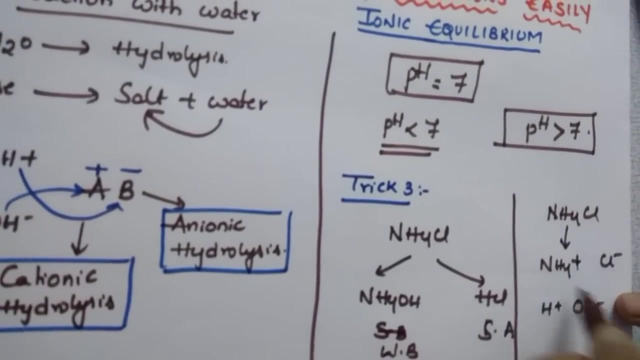 strong base like NaOH and strong acid like HCl. How to do is: I will tell you a small, easiest method. Suppose NH4Cl. what you do is just break into ions, NH4 plus and Cl minus. Just add water to this. Water dissociates into H plus and OH minus. Plus. charge is there, so it combines. 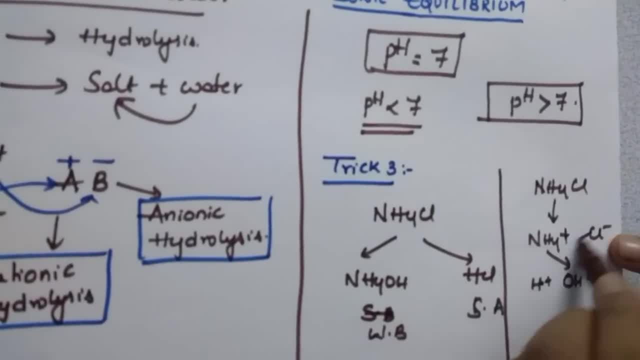 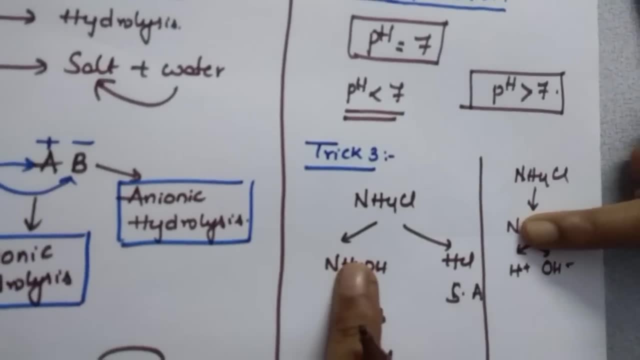 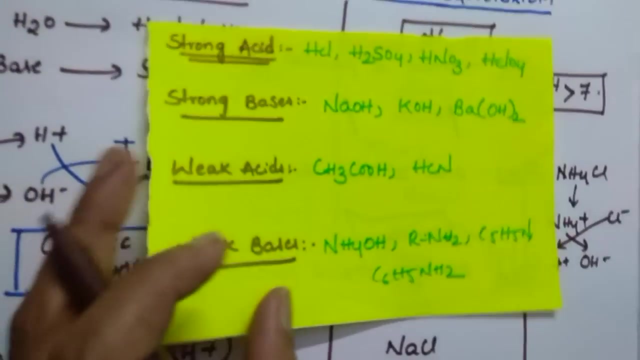 with OH minus- and here plus charge is there- it combines with Cl minus. It forms NH4OH and HCl. So NH4OH is a weak base and HCl is a strong base. In this way dissociate it and check it out. Still, you don't have an idea of strong acid. and 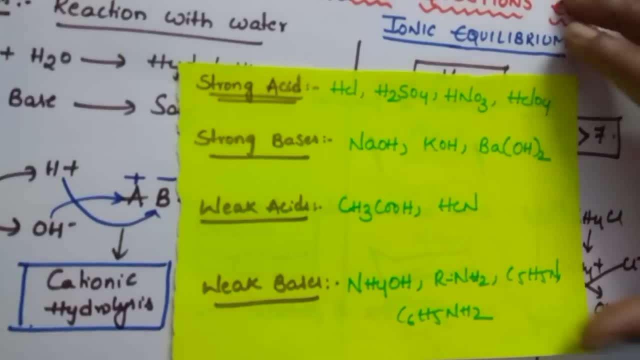 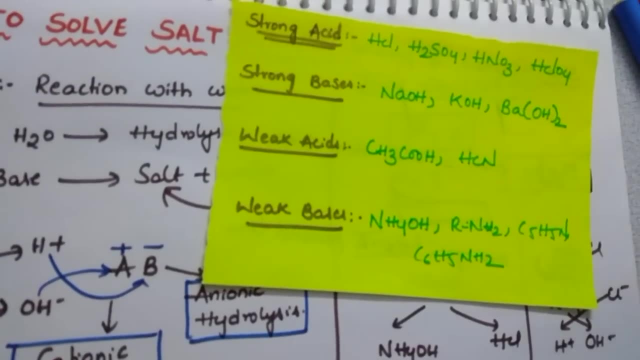 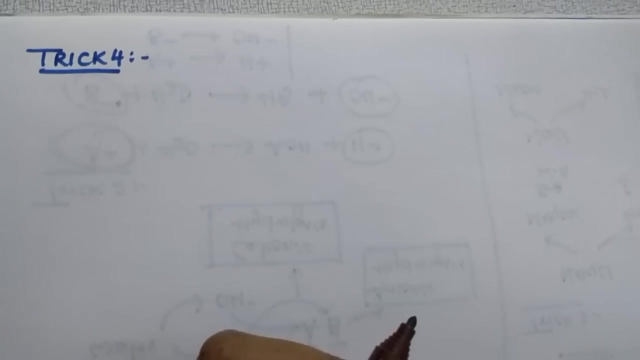 strong bases. then go through this, note down this, and just practice different salts. You will come to know which is in the combination of salt, which is formed from strong acid or weak acid or weak bases. Trick number four. Trick number four. See, students just understand the difference. 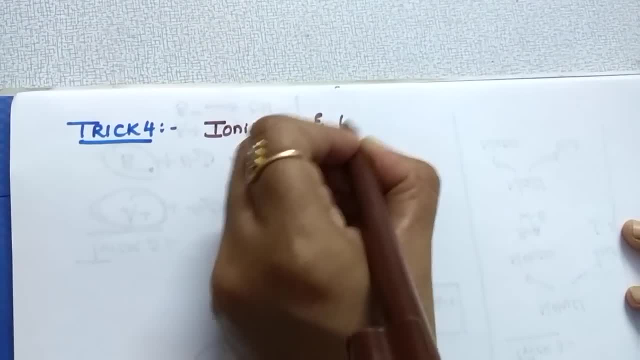 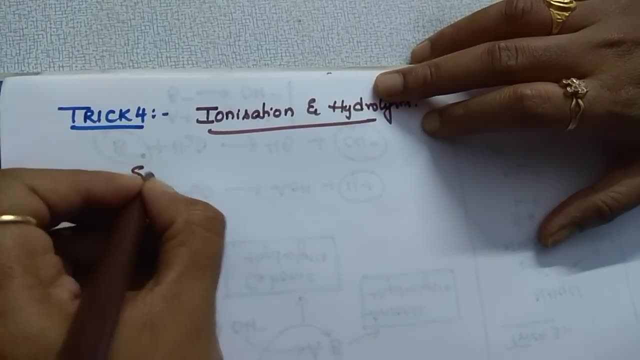 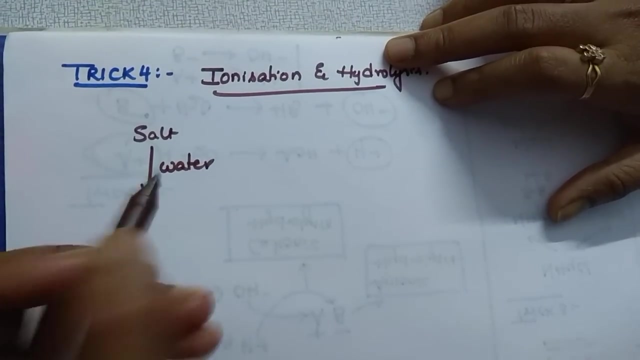 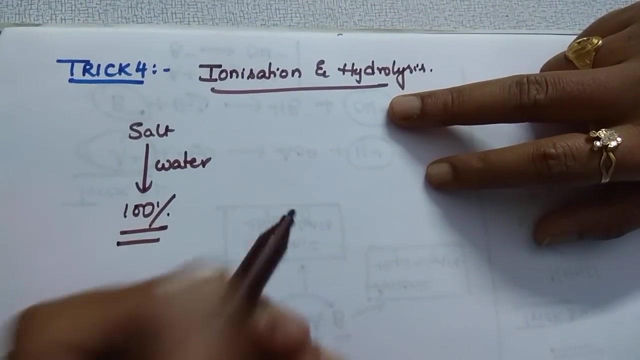 between ionization and hydrolysis. Ionization in the sense, suppose, if you dissolve a salt in water, salt in water, it dissolves, It dissociates into cation and anion and it dissolves in water. Then if it completely dissolves, we call it as this salt is 100% as ionized. and let us see the. 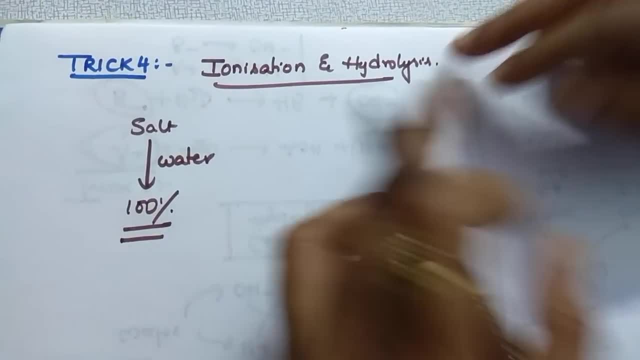 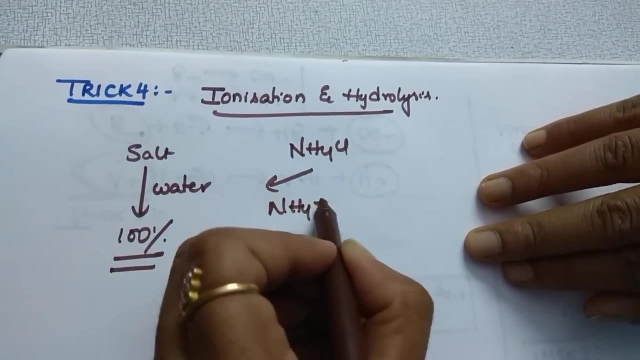 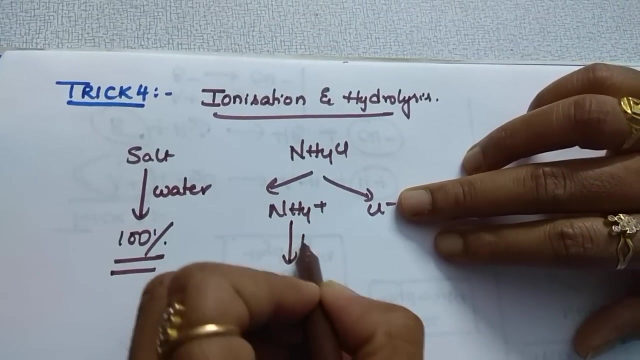 hydrolysis means whatever the ions are dissolved, in that it has to react with water. Suppose, if you see NH4Cl, it dissolves in water and breaks in. it breaks as NH4 plus and Cl minus. but this is called ionization, Whether it reacts with H2O or not. if it reacts with H2O, 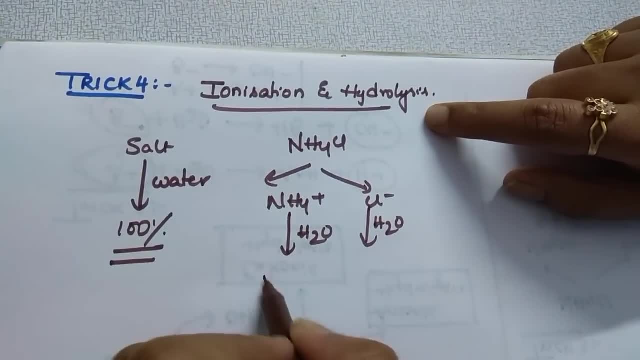 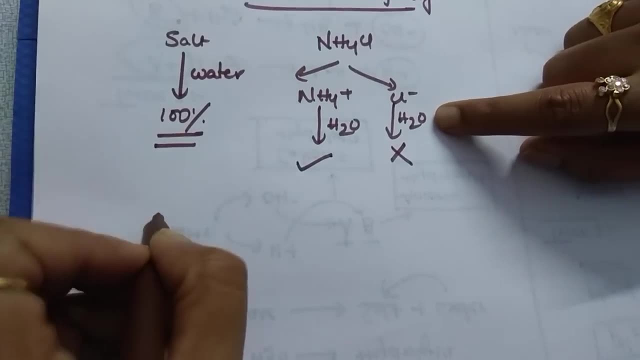 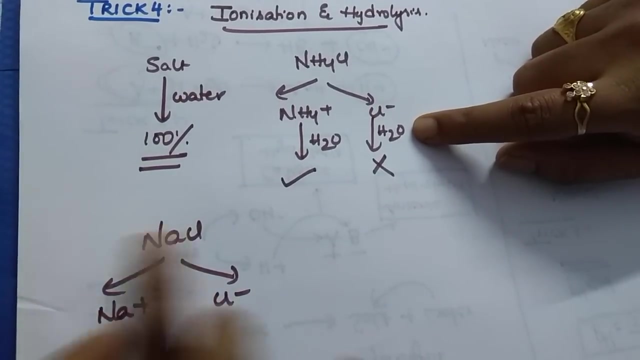 then we call it as an hydrolysis. Here NH4 reacts with water, NH4 plus reacts with water, whereas Cl minus won't react with water and if you see NaCl, it dissociates to Na plus and Cl minus. This is called as when you dissolve in water, this is called ionization. 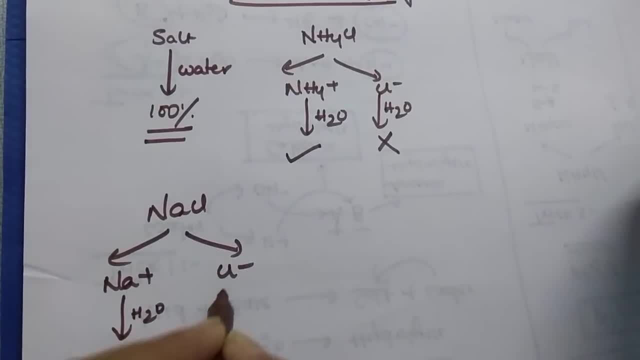 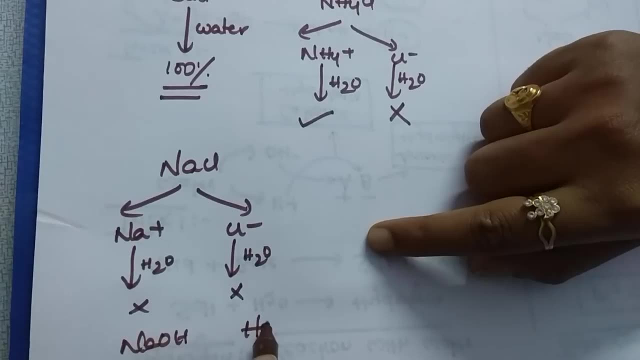 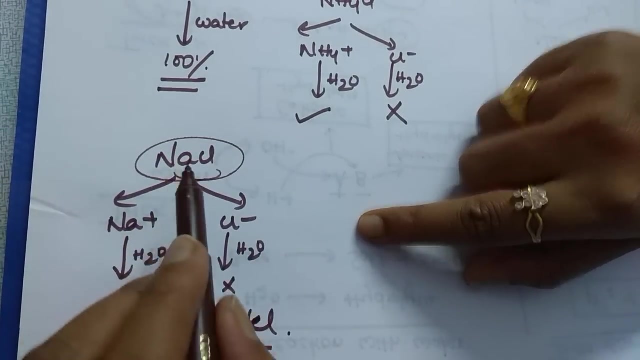 but whereas Na plus do not reacts with water and Cl minus do not reacts with water, If it reacts with water, it forms NaOH. If it reacts with water, it forms HCl. So when you dissolve salt in water, you won't get NaOH and HCl. This NaCl won't undergo hydrolysis. It undergoes only. 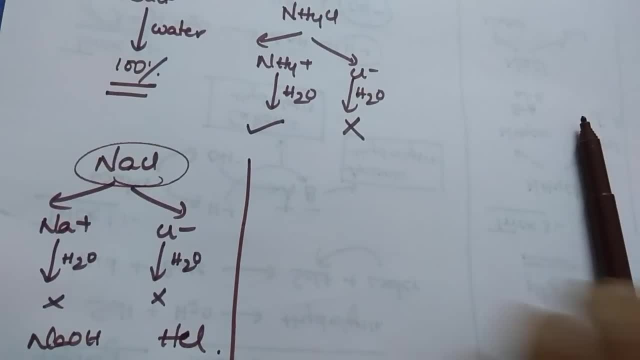 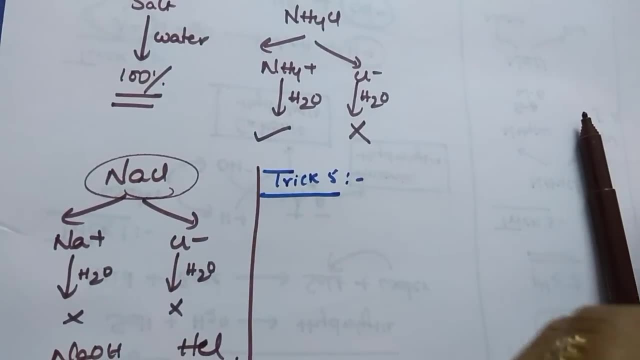 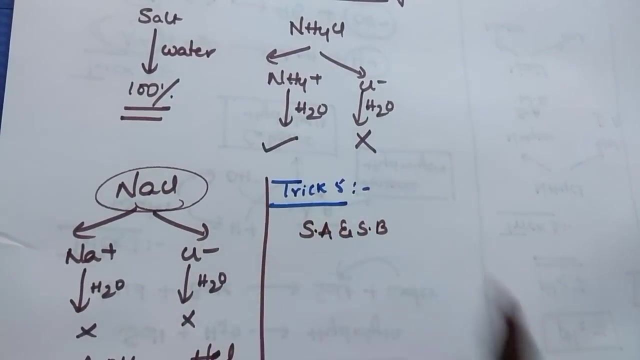 ionization. So let us see trick number five. Which one undergoes a hydrolysis, Which one won't undergo hydrolysis? Trick number five: I'll tell you a small point: The salt of either strong acid or a strong base, If any one component in a salt, if it is strong, then it 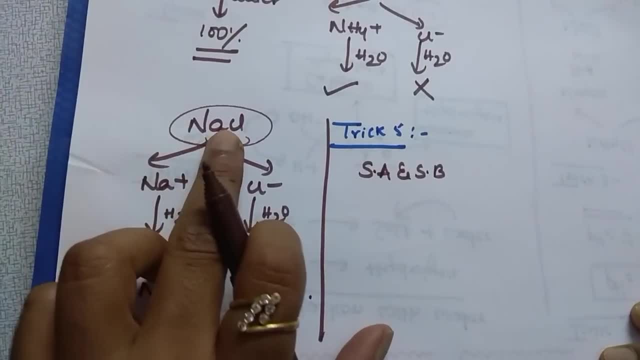 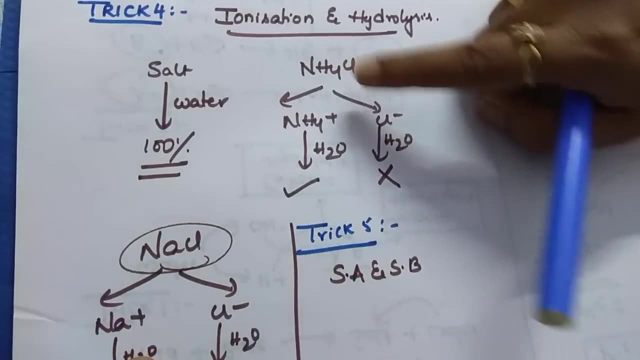 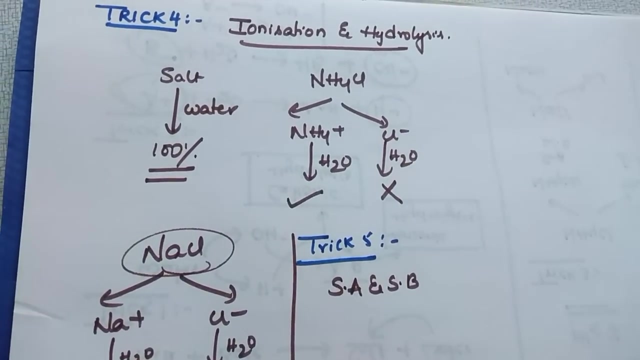 won't undergo any hydrolysis. If you see here, NaCl is formed from a strong base and a strong acid. That's why these ions won't undergo hydrolysis. If you see here NH4Cl- this Cl minus from HCl, That's why it won't undergo hydrolysis. Follow this one, you won't get any confusion. 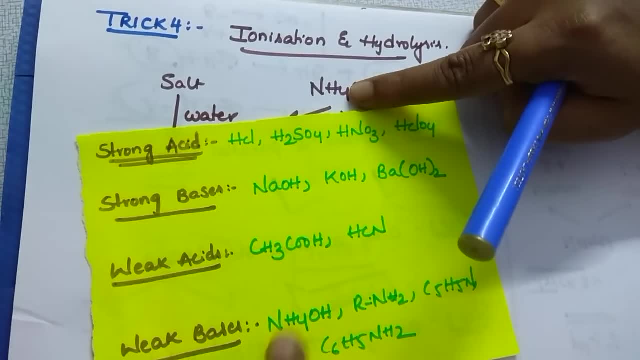 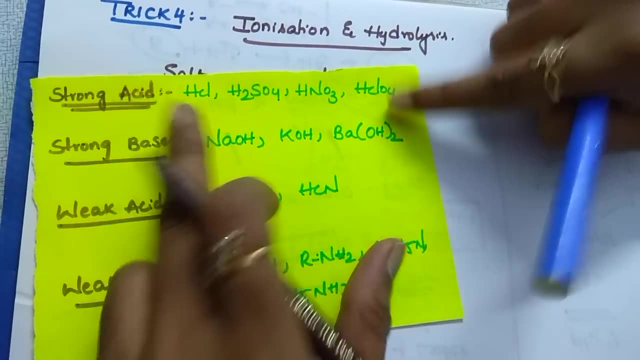 Break this and add to this OH minus, you will get NH4OH. It is a weak base and Cl minus means if you add H plus to that, you will get HCl. That is a strong acid. In such a way you calculate it. 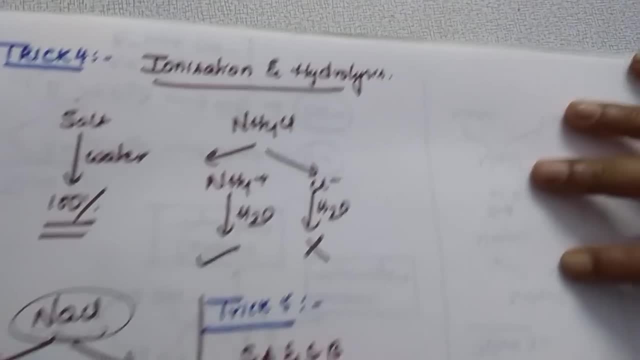 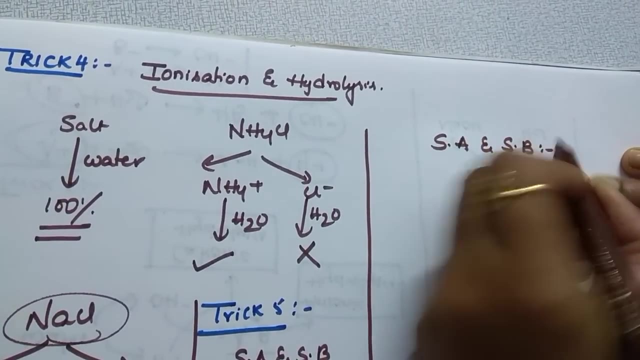 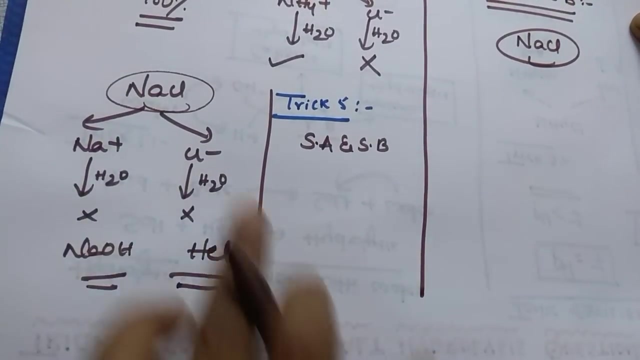 Now I'm going to teach you about salt hydrolysis. See here: strong acid and strong base, like the salt, which is formed from strong acid, And a strong base, like NaCl. if you dissolve in water, it won't undergo any reaction with the 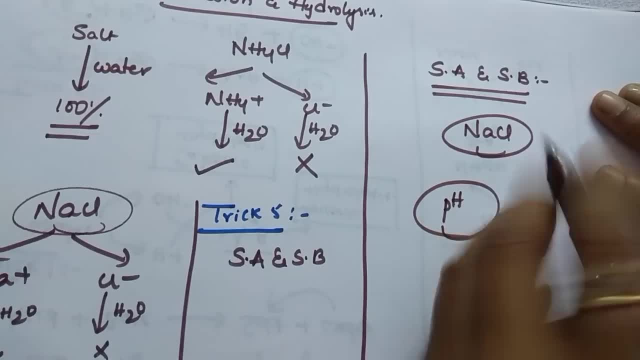 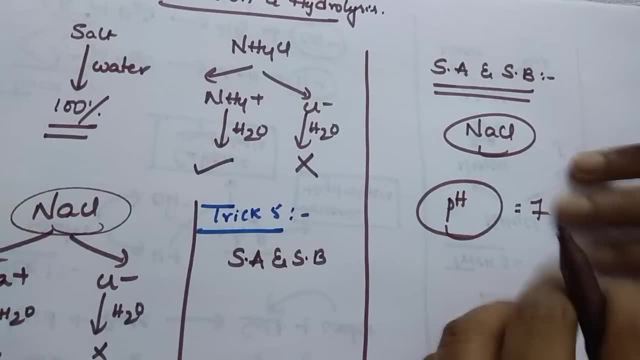 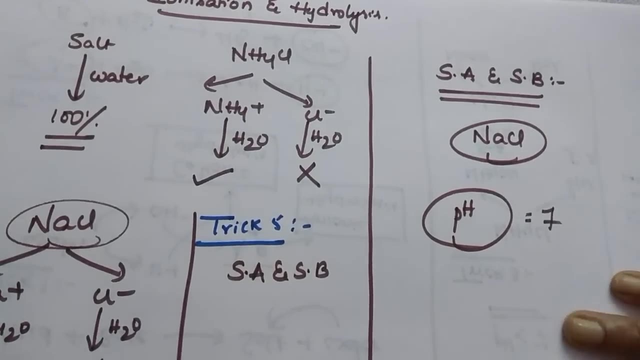 water means after adding the NaCl and or before adding NaCl. Before adding NaCl, pH will be 7.. But after adding NaCl also, pH will be 7.. There will be no change in the pH for the salt of strong acid and a strong base. Now I'll give you some examples. You tell me. 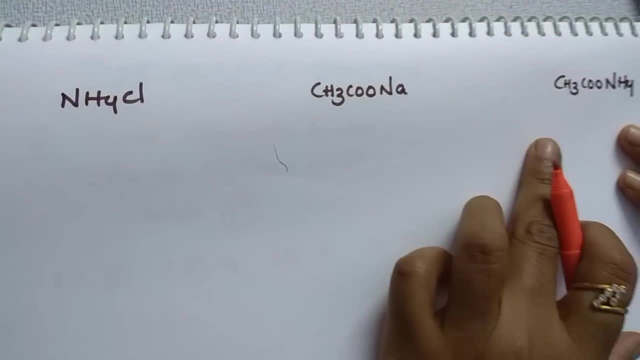 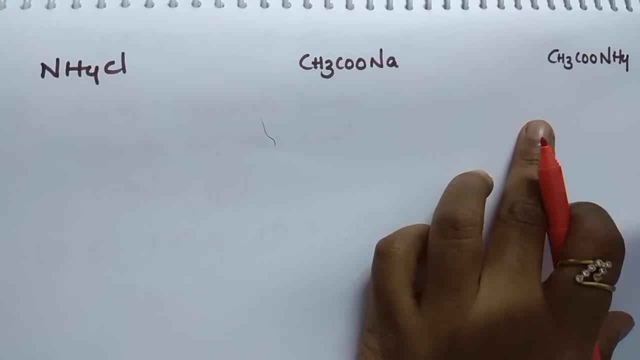 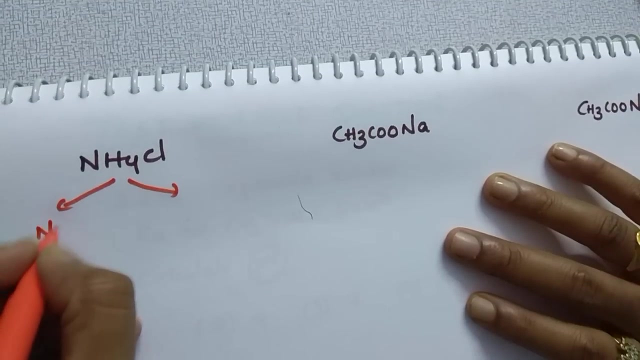 See, students, these three examples I took. Just go through this video and definitely whenever you solve this concept questions, you feel really comfortable and you can solve very easily in a short time. See NH4Cl: it dissociates into how NH4 plus and Cl minus In the same way. 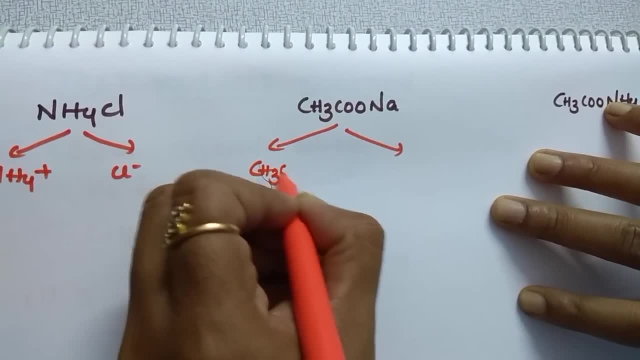 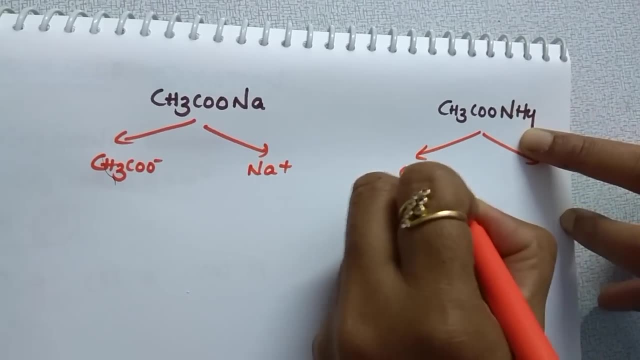 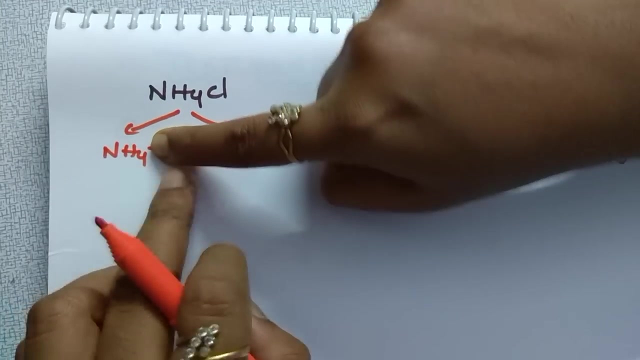 CH3CONa. how it dissociates CH3CO minus Na plus And how it dissociates CH3CO minus NH4 plus. Just add water to this. NH4 plus means OH will come, OH minus, So NH4OH. 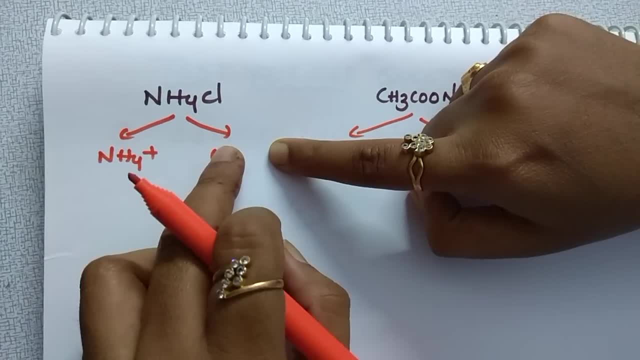 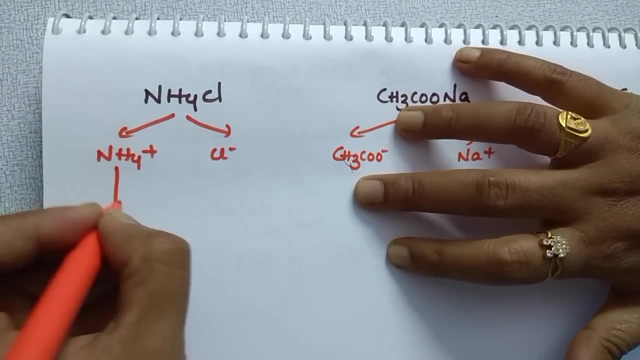 is a weak base. Cl minus means H, plus will come from water, HCl. it is a strong acid In such a way you should do. This is formed from weak base, So weak base is always weak, always undergoes. 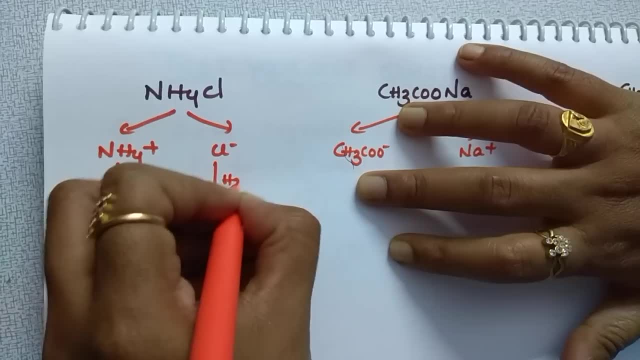 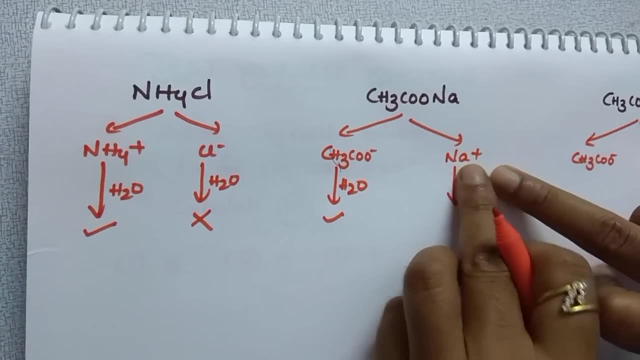 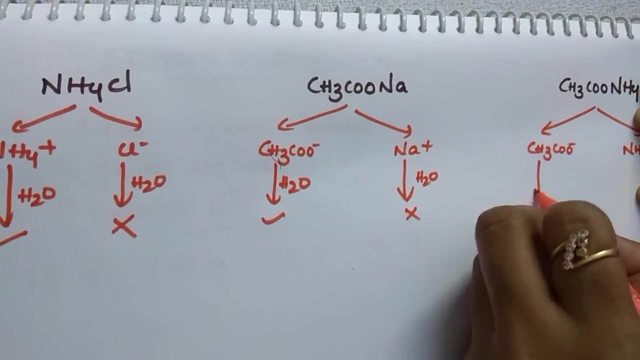 reaction with water. Whereas the strong water I taught you, it won't undergo any reaction with water. Here it undergoes reaction with water, Whereas it is formed from is formed from weak acid. It is strong base, So it won't undergo any reaction with water. This is important. It will, and both 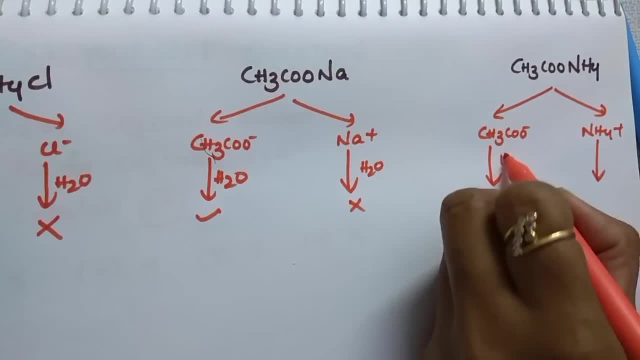 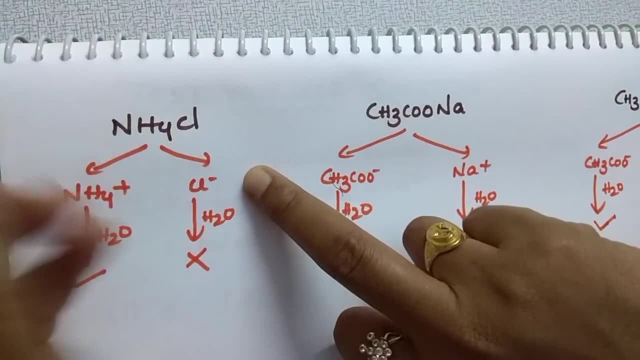 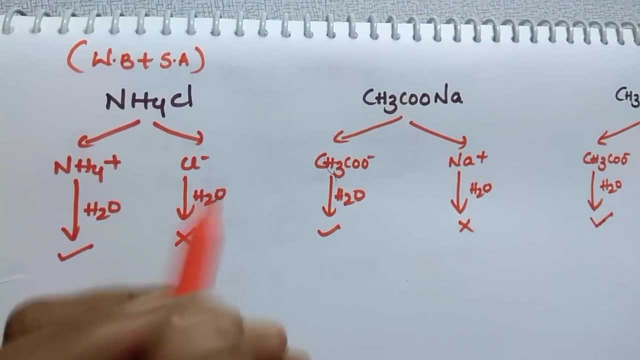 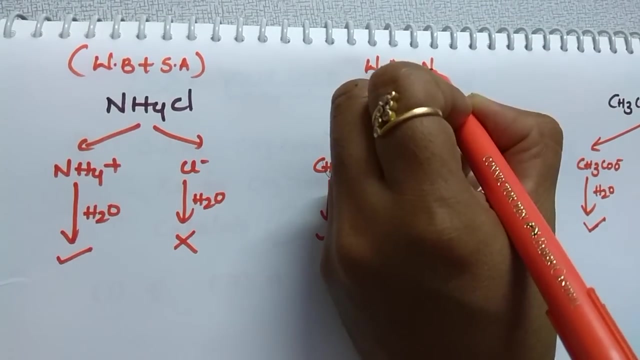 are weak, So this is reacts with water and this is also reacts with water. Clear What I taught you. this is formed from weak base and strong acid. NH4Cl is a salt of weak base and strong acid: CH3CO- weak acid- CH3CONA- weak acid and strong base. This is weak acid as well as weak base. 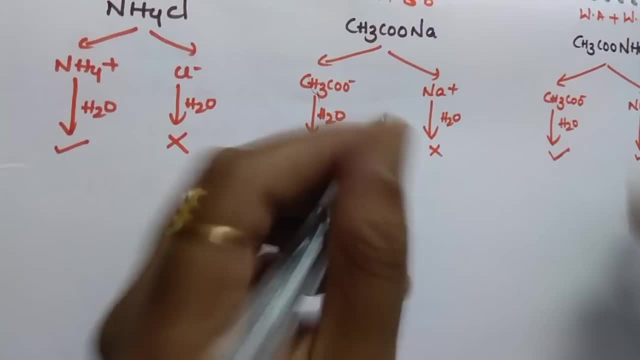 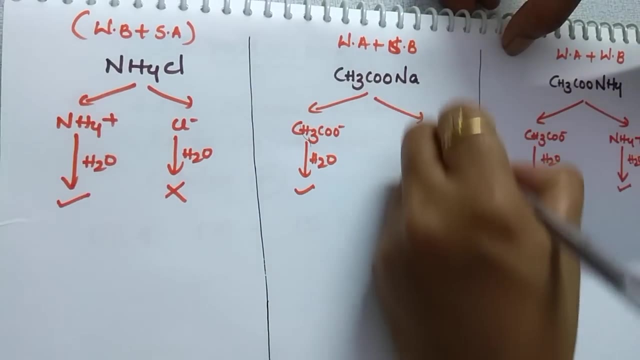 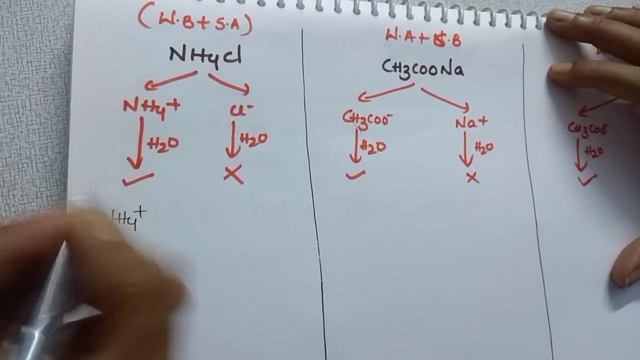 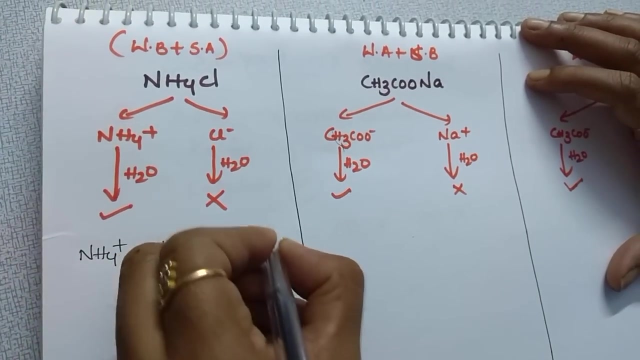 Now see, students, I am going to write the reaction. Just write the reactions. You also take your chemistry booklet and write down Chemistry books. See here: NH4.. Plus, It reacts with water. Which part it reacts: OH minus of water it reacts, and what will be left? 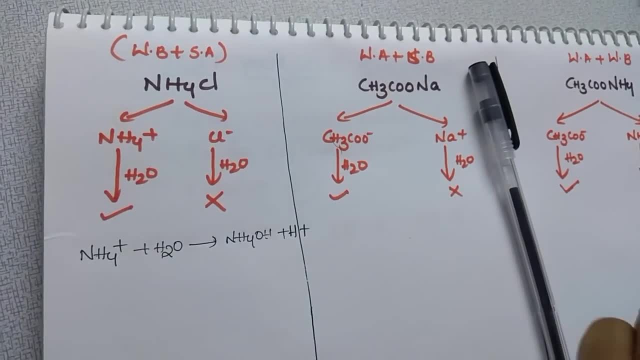 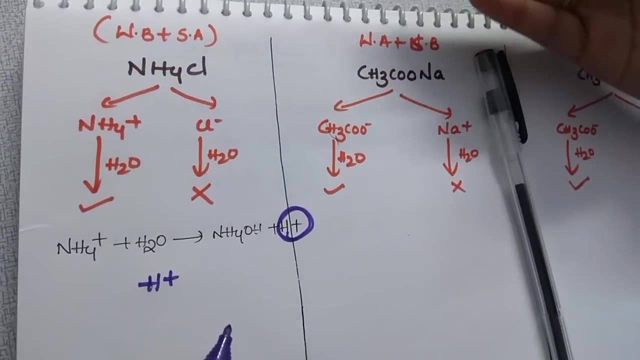 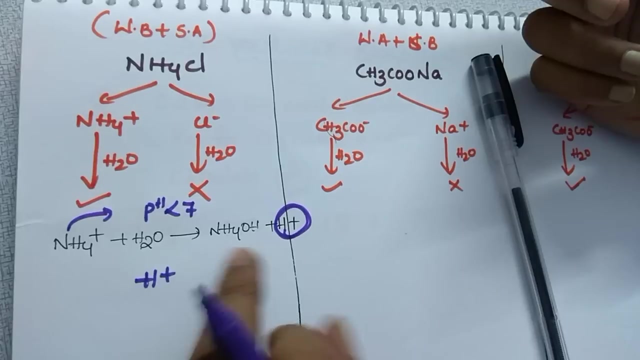 in water H plus is left. So here H plus is left Means whenever H plus ion concentration is left, what happens to the pH? pH will be less than 7.. In whenever a salt of weak base and strong acid. 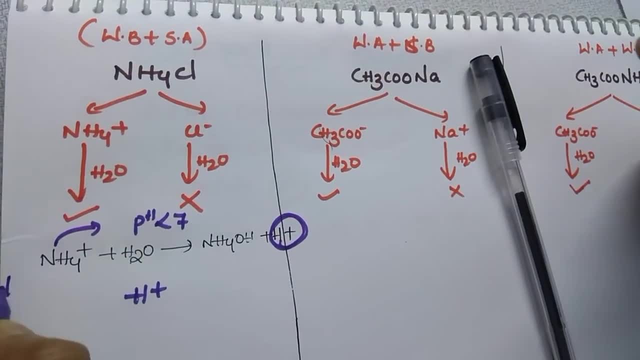 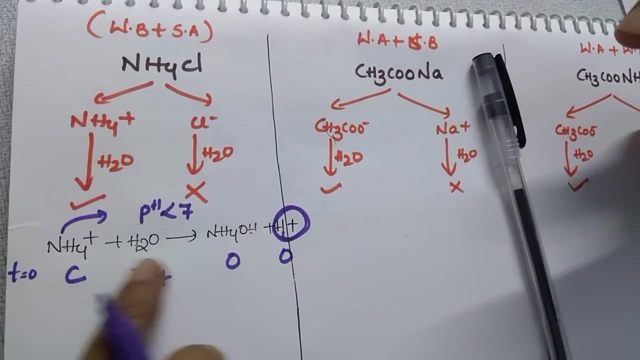 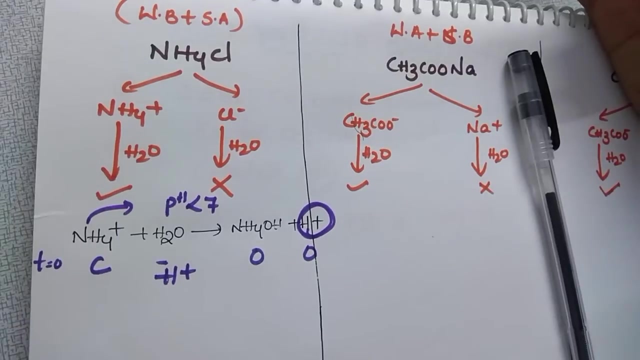 pH will be less than 7.. Suppose reaction is not started, T equal to 0., Its concentration will be C and there is no concentration of products. I take always water concentration constant because it very less amount of salt will be hydrolyzed, So that water large it will be in excess. So 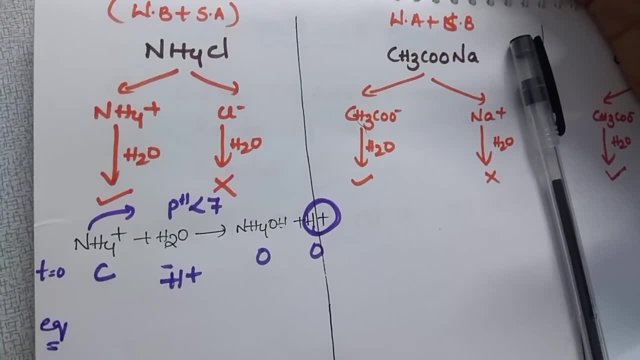 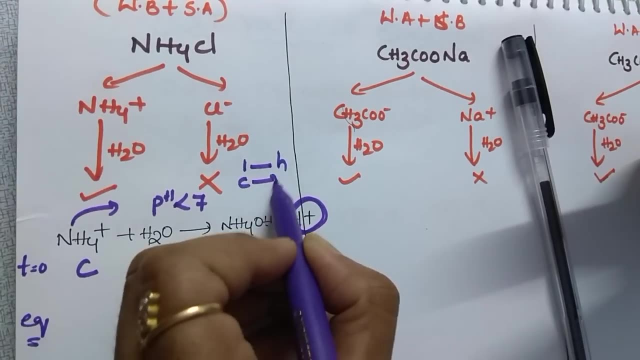 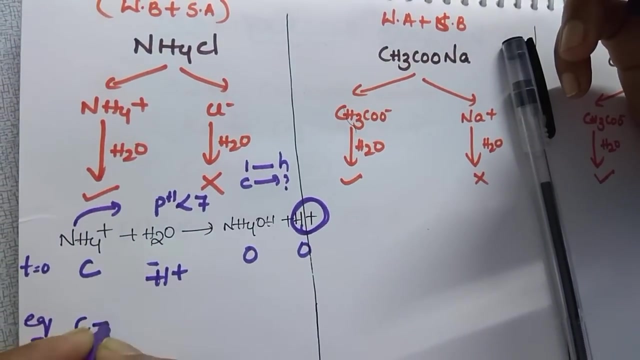 you can take it as a constant, But when equilibrium at a reaction starts, equilibrium stage is reached. for one mole, hydrolysis is H, Then C moles. how much Just do cross multiplication? CH Means amount of salt is hydrolyzed from C, So C minus CH, because CH moles is hydrolyzed from C. and how? 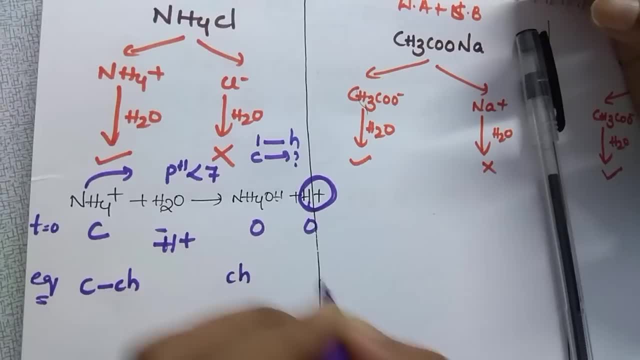 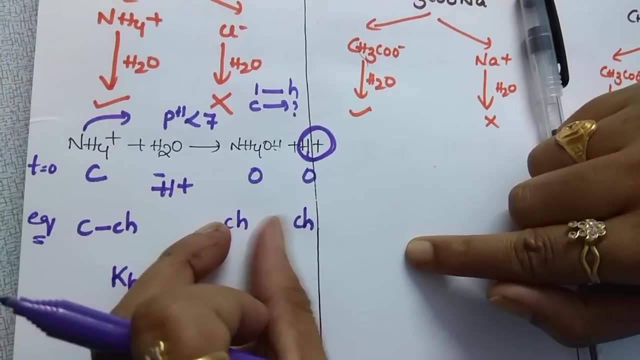 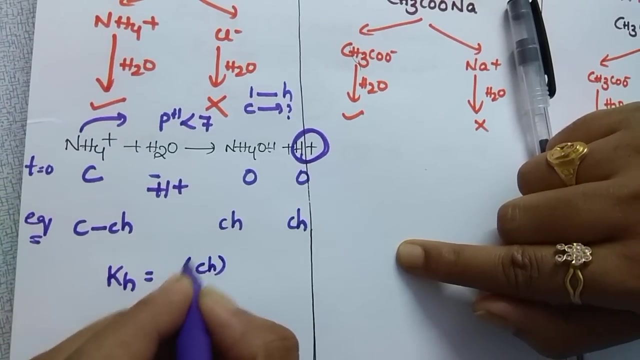 many moles of NH4 OH will be formed CH and H plus how much it will be formed CH. Then how to write hydrolysis constant KH value? It is just the product of concentration of products divided by concentration of the reactant, So CH into CH, divided by concentration of C minus CH. 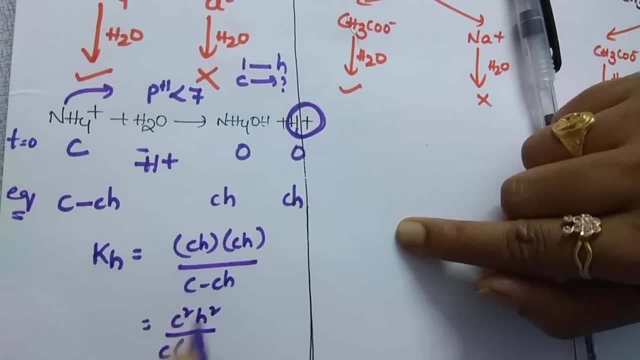 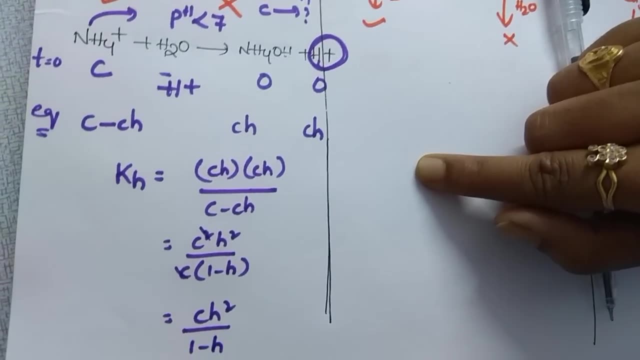 Just C square, H square by C. I am taking common here: 1 minus H, Then this C, this C will be cancelled and CH square by 1 minus H is left. This is KH See students. this is the case where, when, suppose. 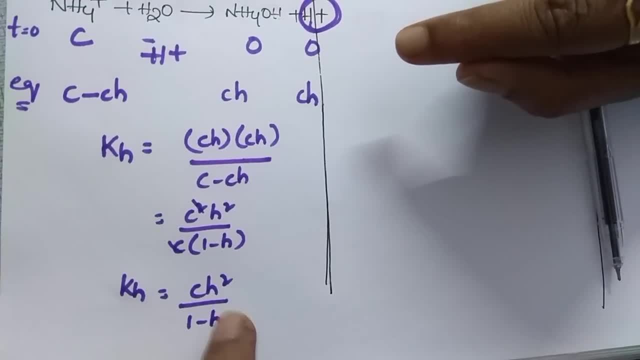 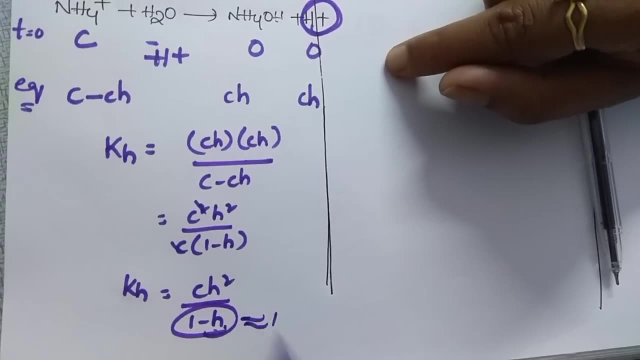 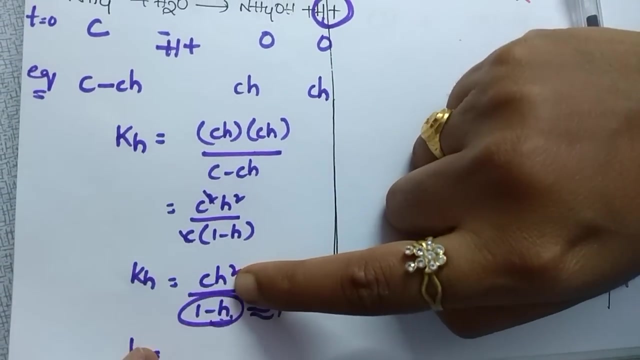 degree of hydrolysis, H is very less. In such a case you can neglect this term. 1 minus H, This is very less. Then you can take it as an almost 1.. Then KH is equal to CH square, Then H square is equal to KH by C. Then H is equal to square root of KH by C. Clear, This is most. 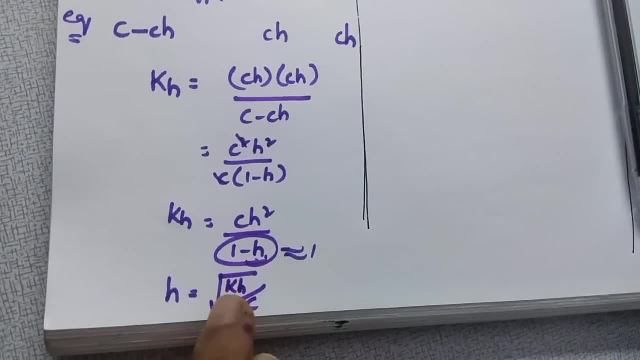 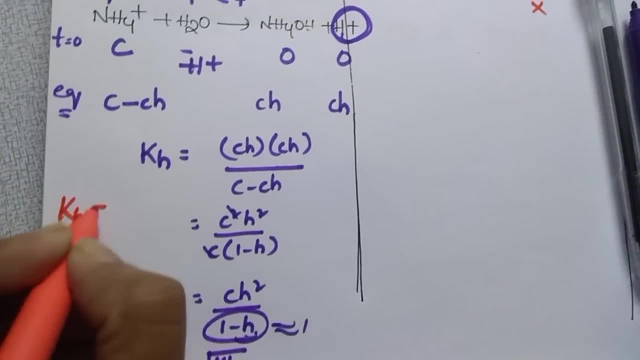 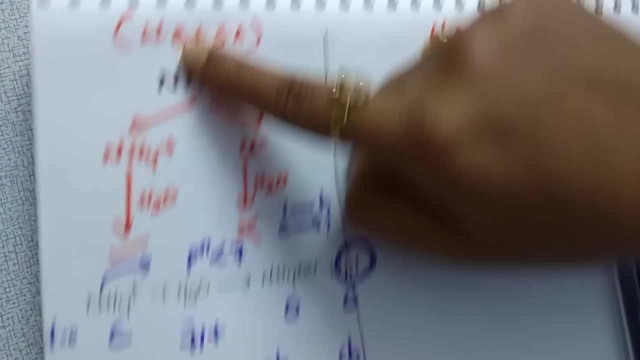 most important, And in your exam they won't give you KH value. You have to calculate KH. How to find KH is KH is equal to KW by ionic product of water divided by See. I will tell you a small trick. It is a weak base, So you have to take KB value down. 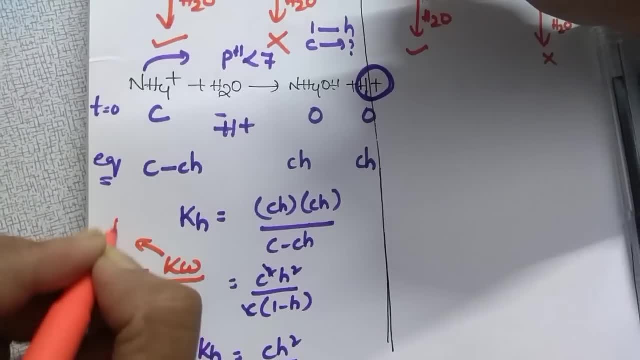 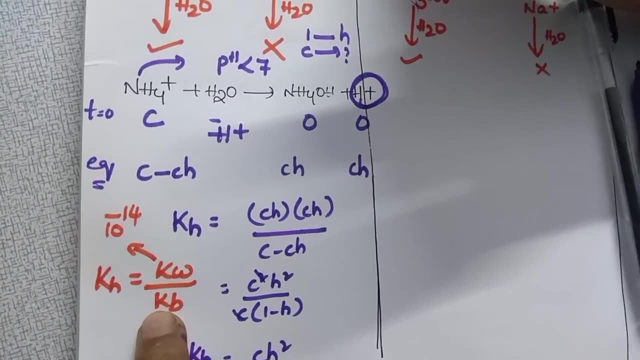 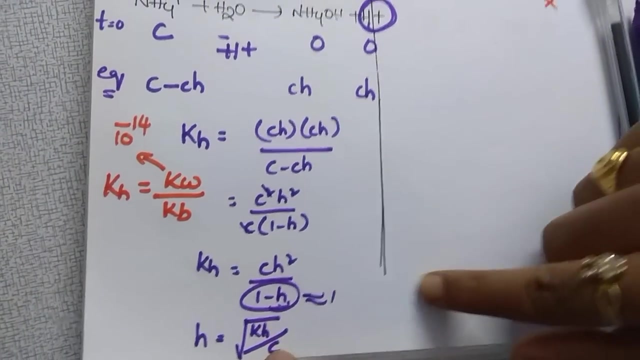 KB value will be given in question. How to take KW. KW is a constant 10 power of minus 14.. Whatever value gives in your question, you have to substitute in KB, Then you have to calculate KH. Once you get KH, then substitute that here and take concentration from the. 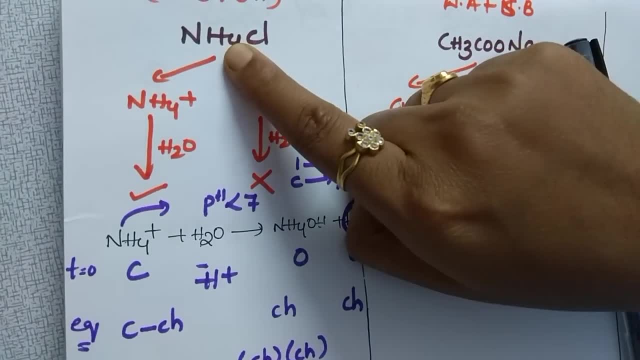 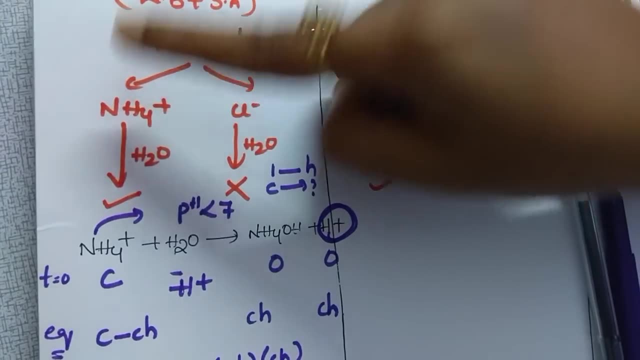 salt of this or how many. Suppose this is 0.1 molar means you have to take 0.1 molar of this one. If suppose this is NH4 twice anything, then it will give this is 0.1 molar. 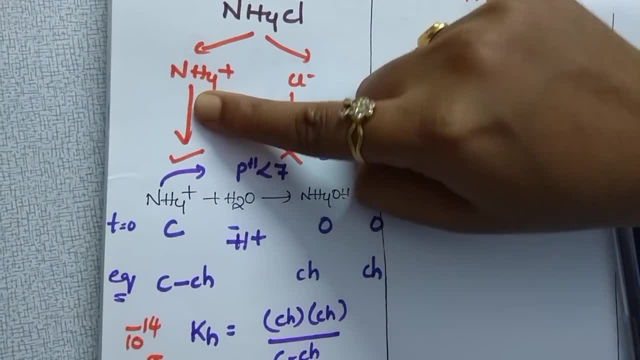 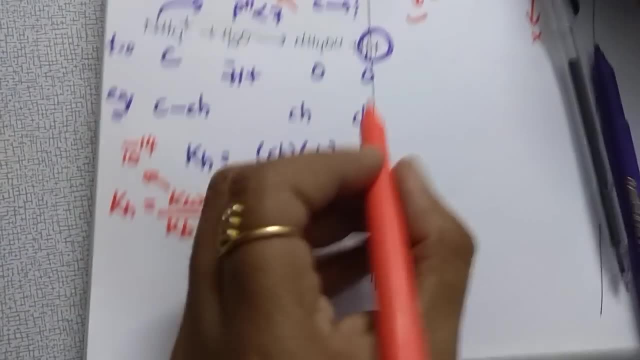 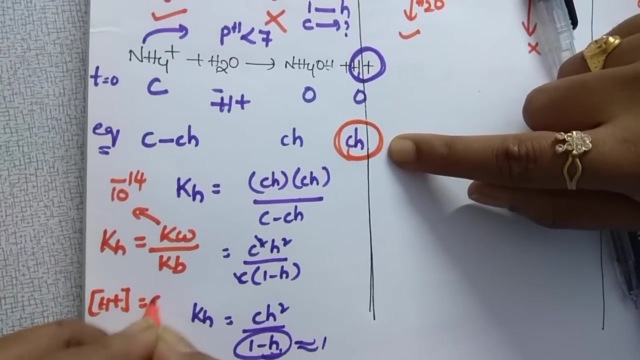 But how many ions it gives 2.. So you should take 0.2 moles of this and substitute in concentration term and find H. Once you calculate H, then you should calculate H plus ion concentration. See H plus ion concentration is equal to what students? CH is the formula Right, C is given. 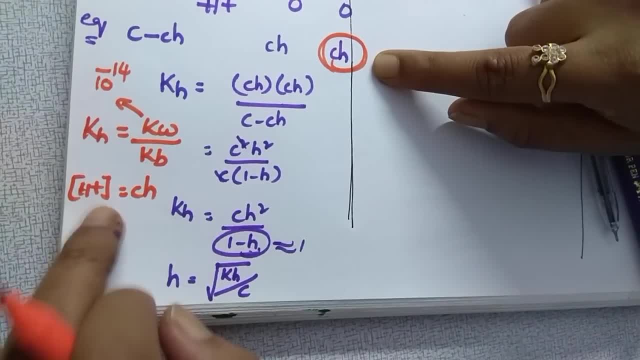 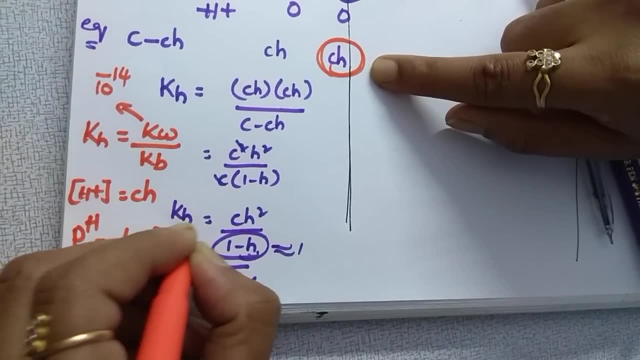 in the question H you calculated here You get concentration of H plus. Once you calculate concentration of H plus, just that you substitute In pH formula, that is, pH is equal to minus log of H plus. Then you will get the pH Clear. 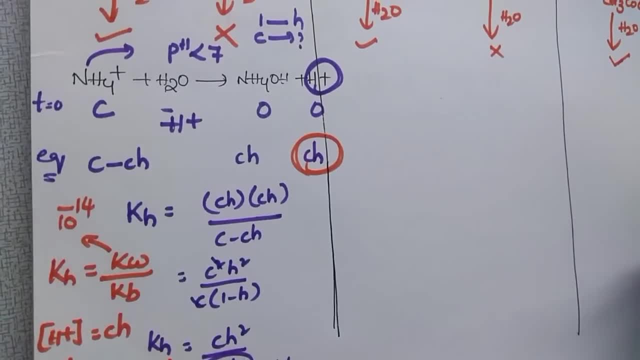 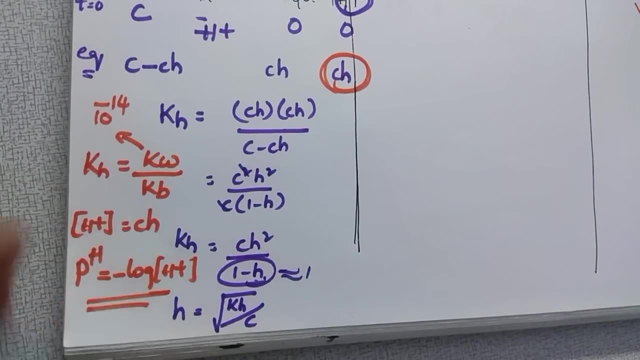 I will give you test yourself question. You don't worry of that. First what you should do. You have to calculate KH, Then you have to calculate H, Then you calculate H plus ion concentration, Then pH. These are the four formulas. Next, in the same way, if you 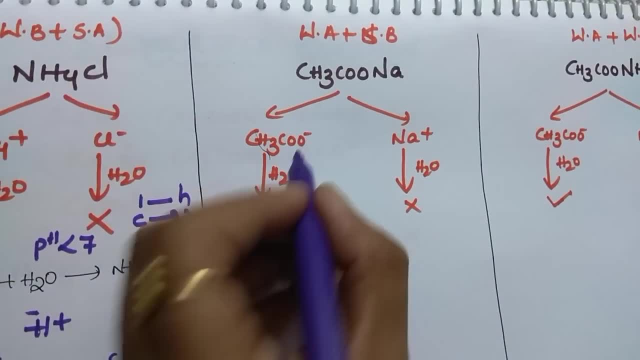 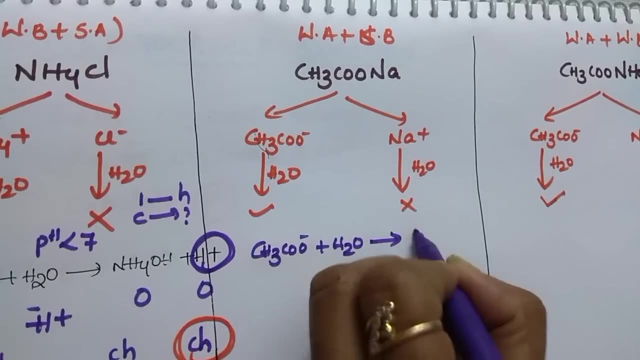 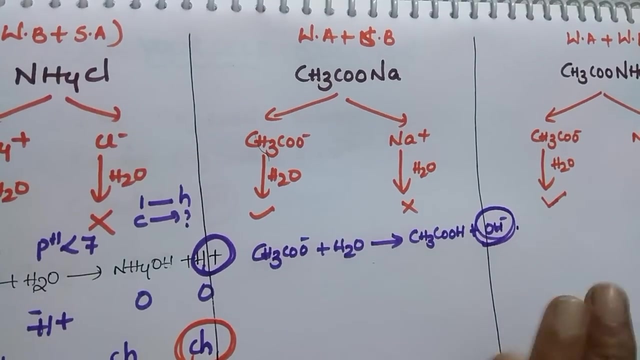 do the hydrolysis for this anion? what is that CH3COO minus? If it reacts with water, what do we get? CH3COOH plus, OH minus Means it gives OH minus and concentration. So pH will be greater than 7.. Right Now, when reaction is not started, its concentration 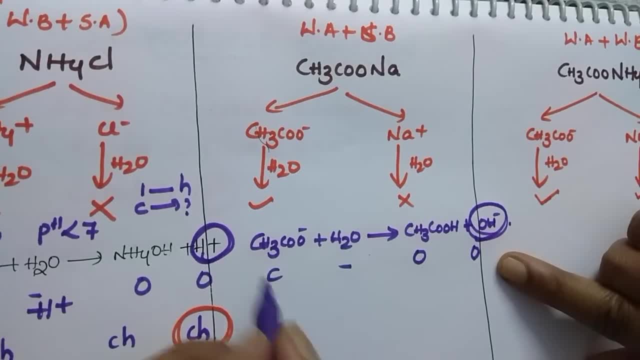 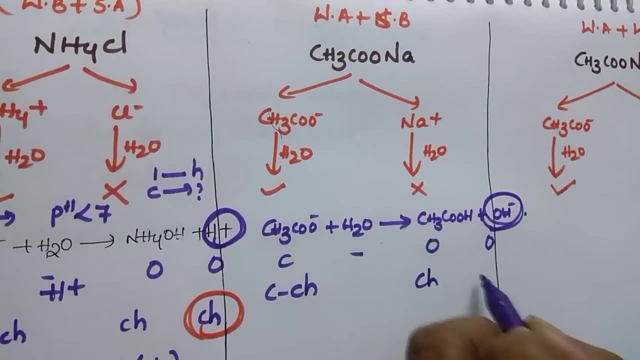 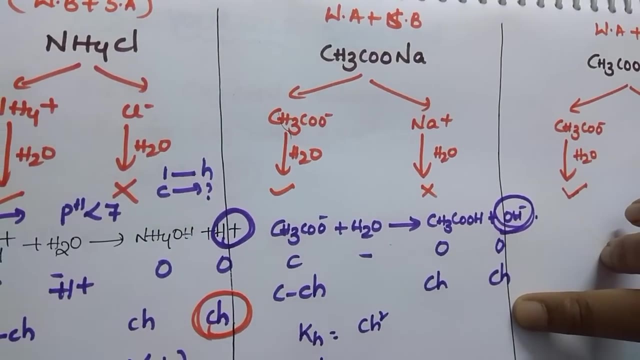 is C and no products. When reaction is started, degree of hydrolysis, CH means CH moles is dissociated from C, Then it forms CH. Same way, if you do KH, same way, you get this formula: Which one CH square? Then H will be square root of KH by C. I am not doing same, You do it, you. 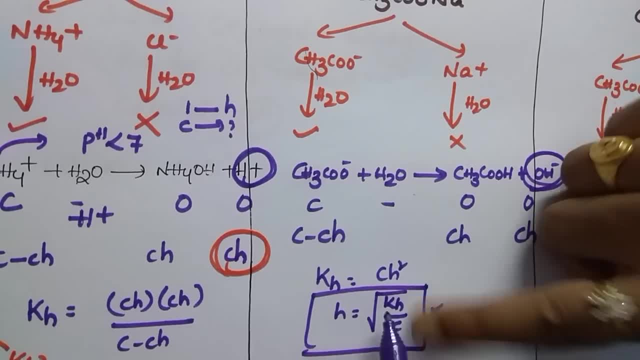 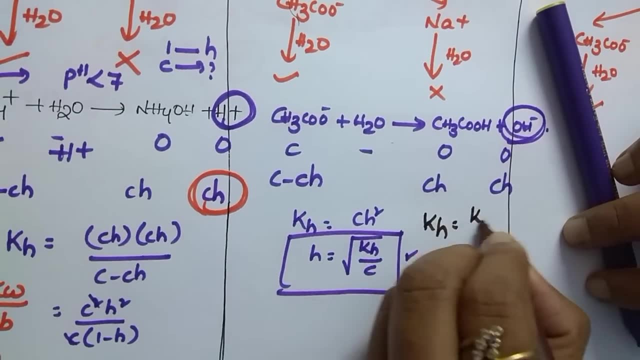 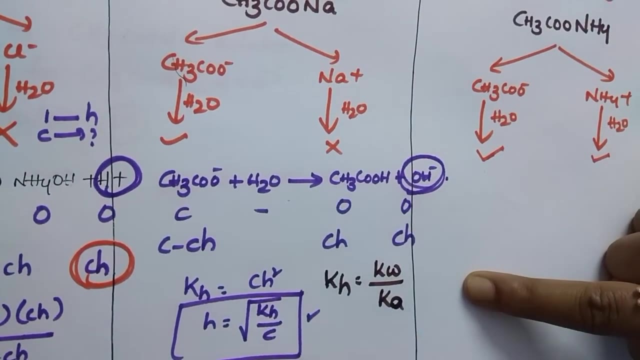 will get the same thing. This is the most important formula: KH you won't. they won't give in question. You have to calculate How to calculate KH. KH is equal to KW by K, A or B. Here it is a weak acid salt, So you should take K. It will be given in question. 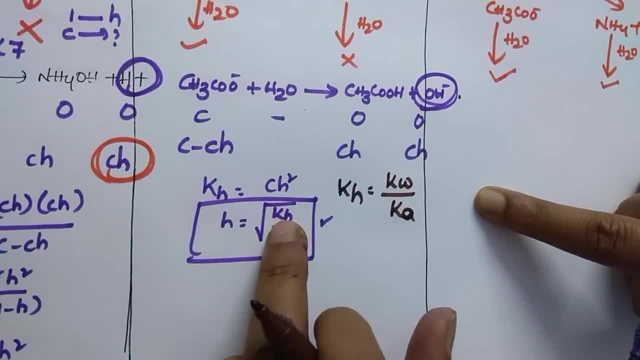 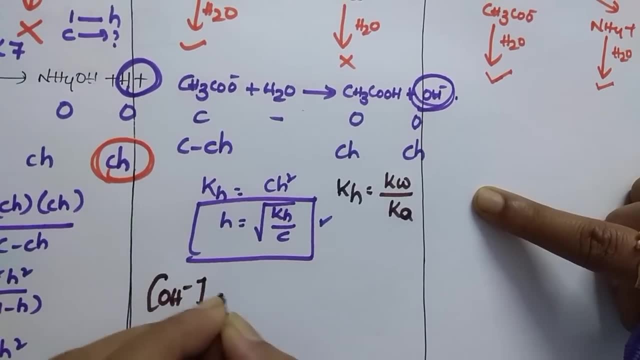 Directly substitute it. Get KH. That KH substitute here and concentration will be given in question. You will get a H Once you get H here. what students do mistake is they think that it is H plus sign. concentration is equal to CH. They substitute and they will calculate pH. 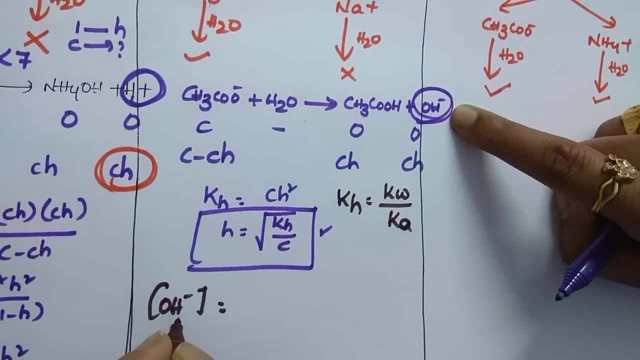 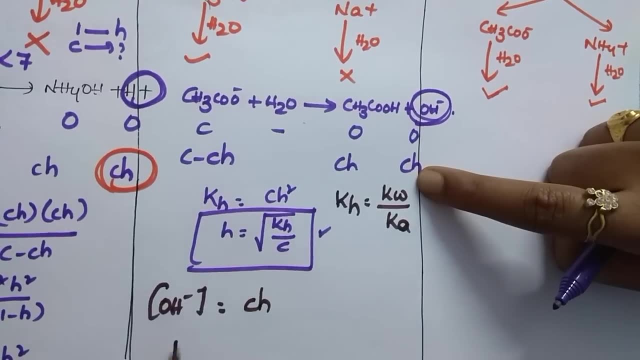 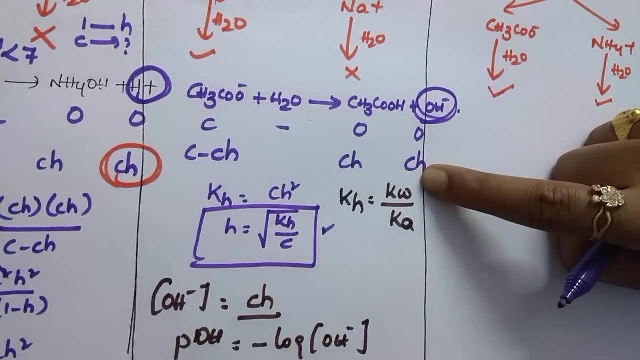 But what you get? OH minus. So OH minus sign concentration is equal to what is that CH? Substitute that H here, Then POH is equal to whatever the value you will get. minus log of that concentration you take, you will get POH. 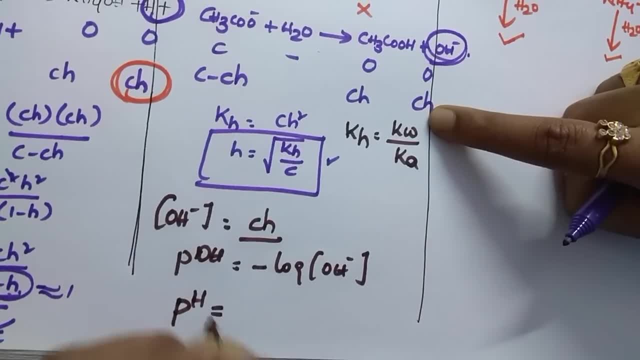 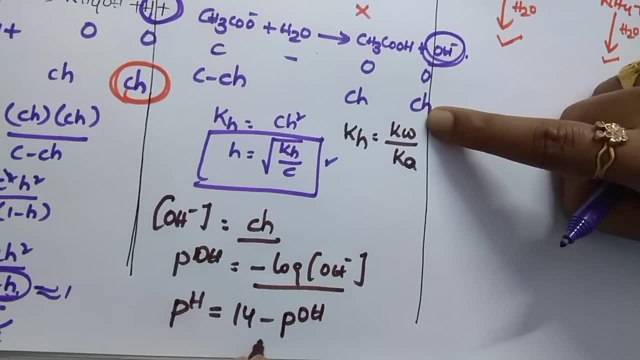 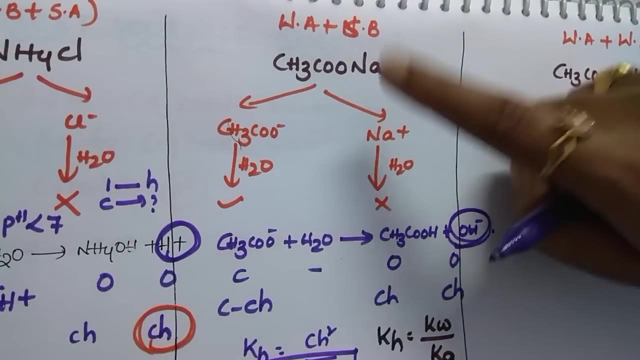 Once you get POH, then pH is equal to 14 minus POH. Directly. substitute this value, Don't solve here, Substitute here and then solve it. You will get the pH. This step is important: First OH, then POH, then pH. This is for which one Weak acid and strong base, because you 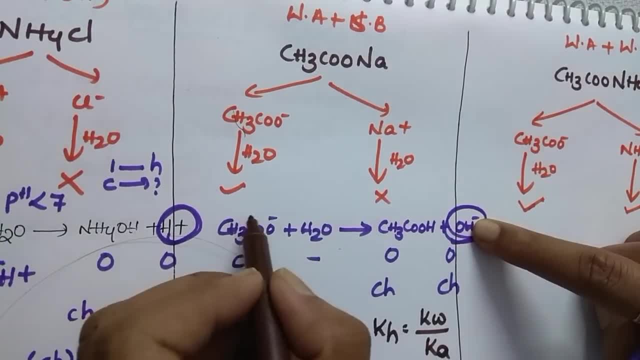 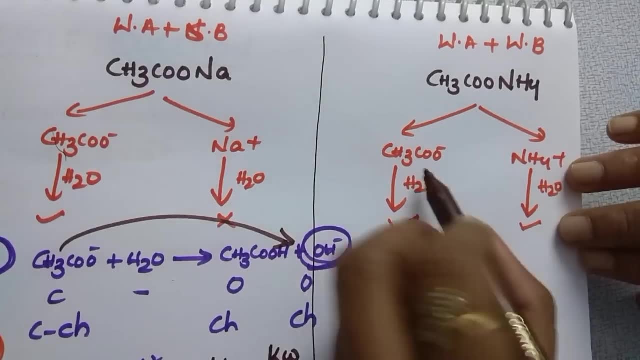 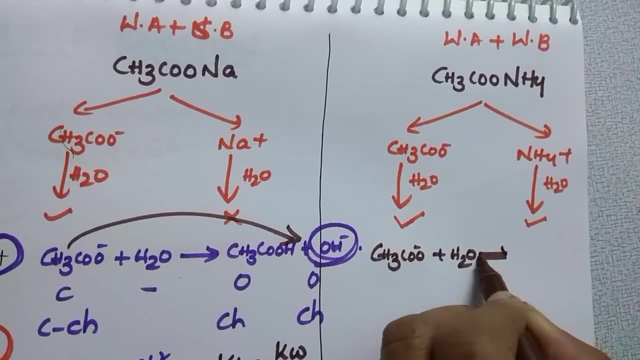 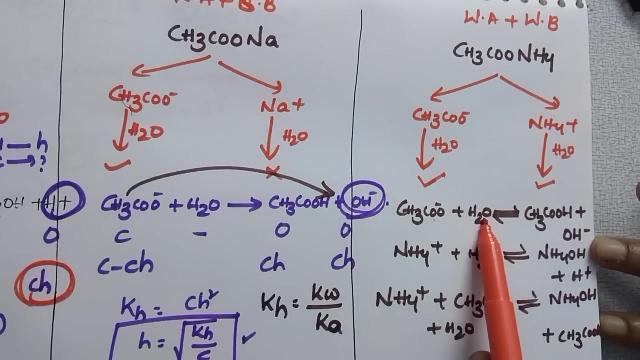 are getting OH minus. If you get confused in your exam, always think anion gives anion. Here it is somewhat little different. Second: here this CH3CO minus reacts with water. See, here I wrote the reaction. Just I wrote how anion reacts with water and forms acetic acid. Here cation reacts with water. 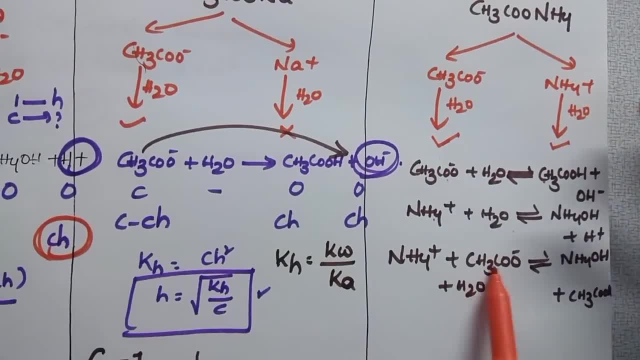 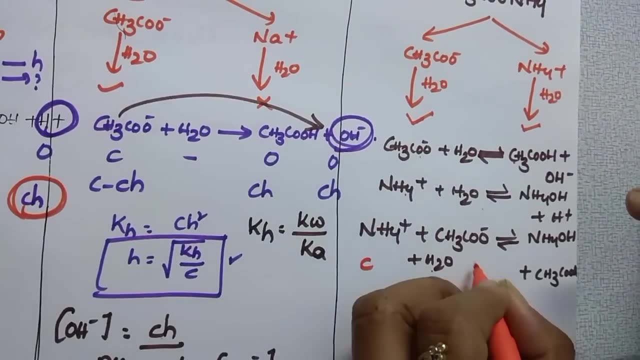 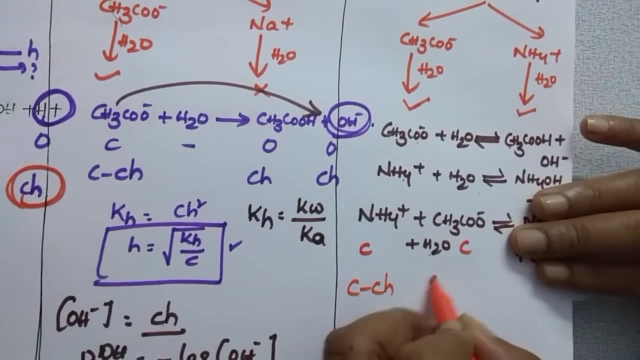 forms a weak base, Both both reacts, Both cation and anion reacts, and you get these products Just. I wrote here This is at initial, its concentration is C and anion concentration is C and no concentration of the product. But at equilibrium: C minus CH, C minus CH. it. 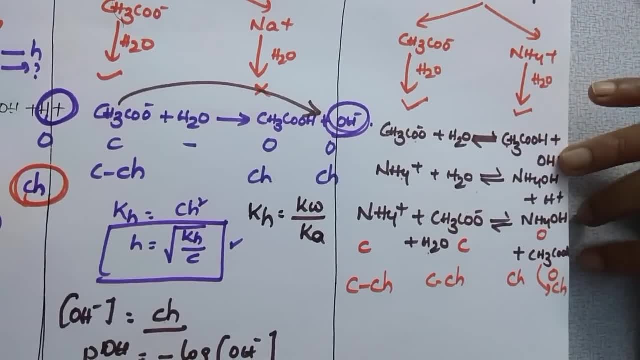 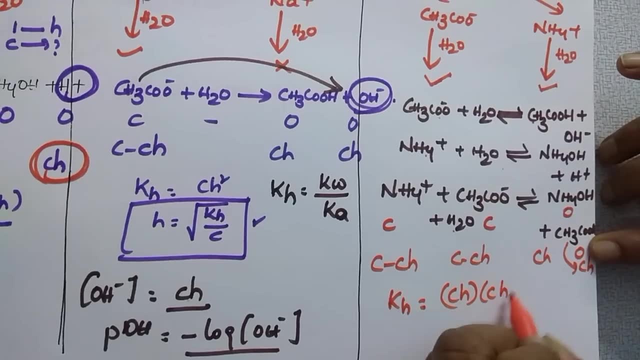 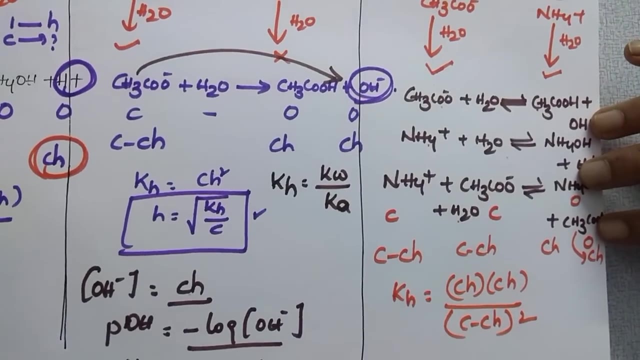 forms CH and CH3COH forms CH. Understand Then how to write K-History: The product of both the concentration CH into CH, divided by both, this into this, Then total C minus CH, whole square. This, upon solving, we get: K-H is equal to C square, H square by C square. 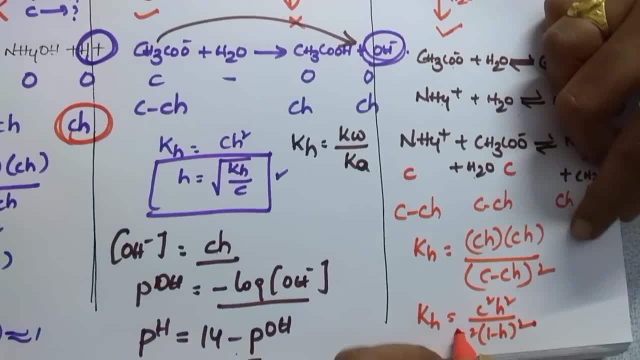 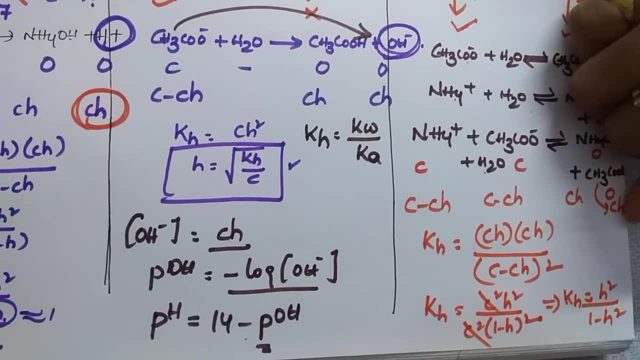 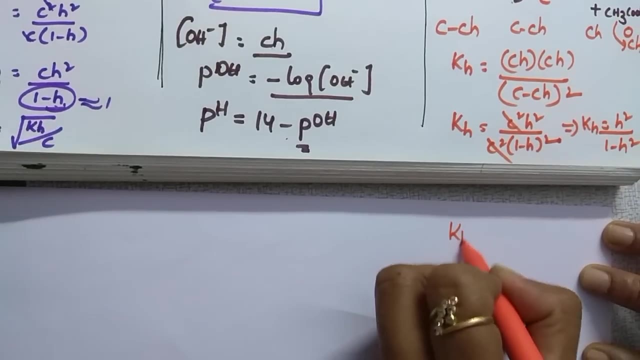 I take common 1 minus H square will be left. So cancel this two. Then we get: K-H is equal to H square by 1 minus H square. Then see here: K-H is equal to what I got: H square by 1 minus H. 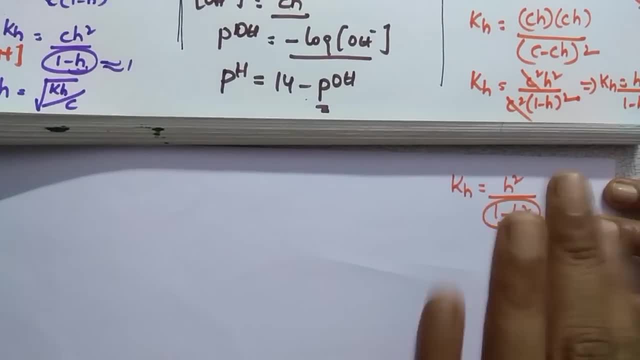 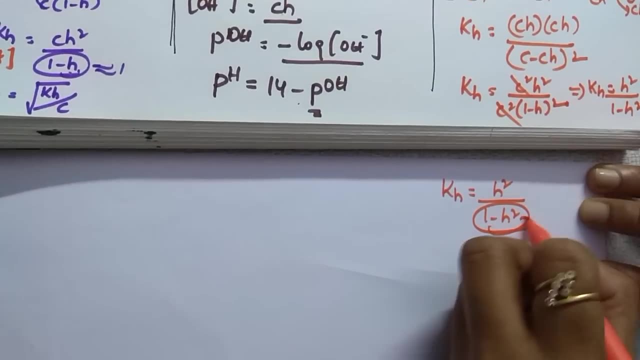 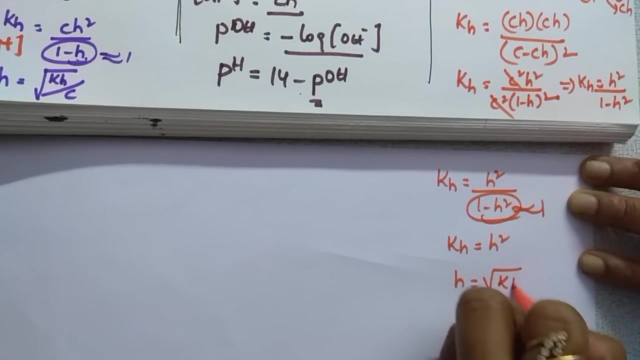 square. Then at whenever, during salt hydrolysis, ionization will be very less, so that hydrolysis will be very less. Take it as almost one negligible. Then we get: K-H is equal to H square, Then H is equal to root of K-H. This is a different formula when compared to remaining to what we discussed. 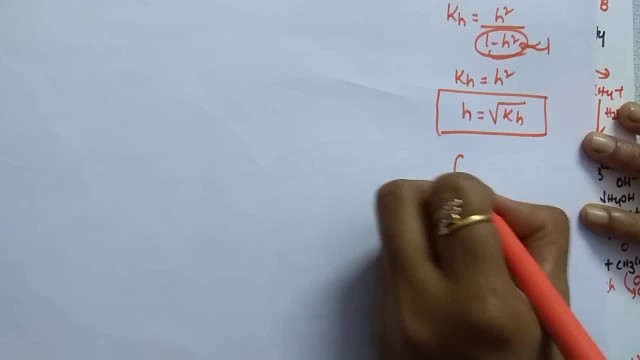 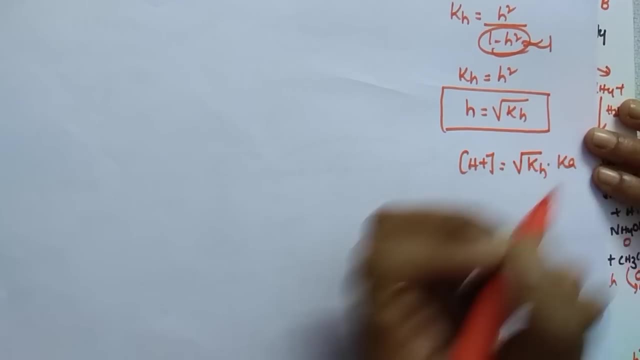 Clear. And once you got this, you have to calculate H plus N concentration. I'll tell you a small formula to calculate: Just multiply this with K-A, You will get H plus N concentration. Once you get H plus N concentration- for this also proof is there, but I'm not discussing. 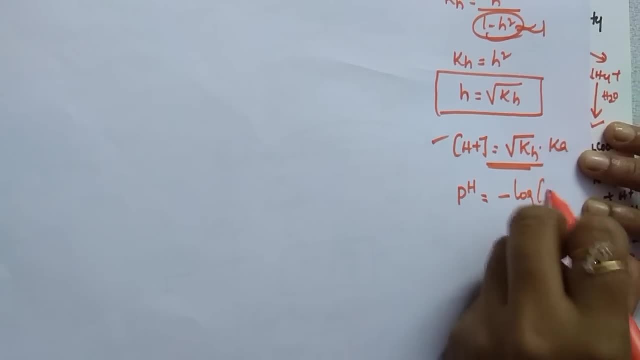 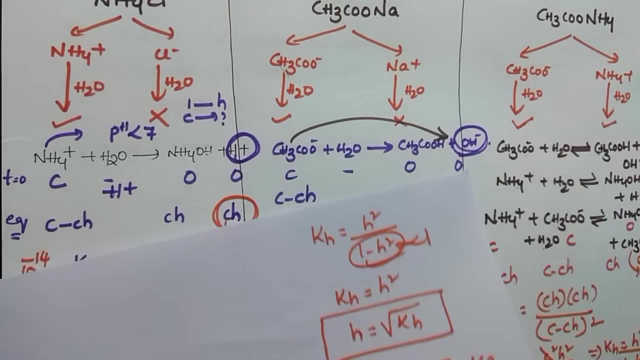 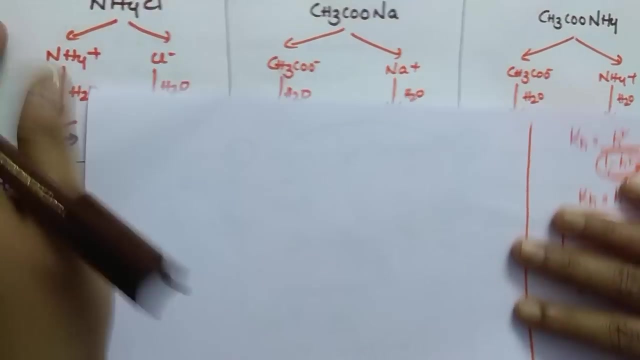 here, pH is equal to minus log of H plus whatever H plus You get here substitute, Then you will get a pH. See, it's a very big concept, but I make in a shot And that is the reason And whether this case known more formula here. 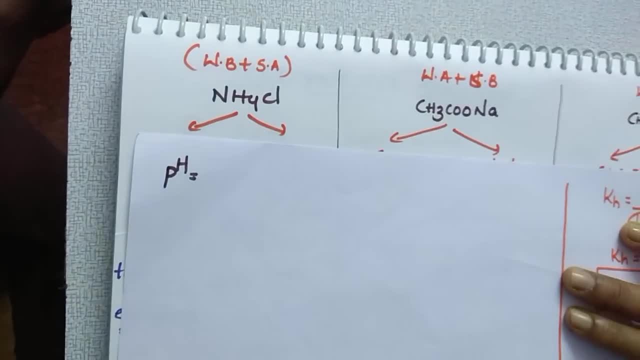 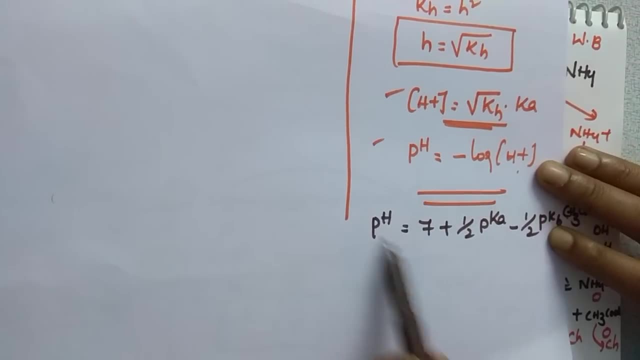 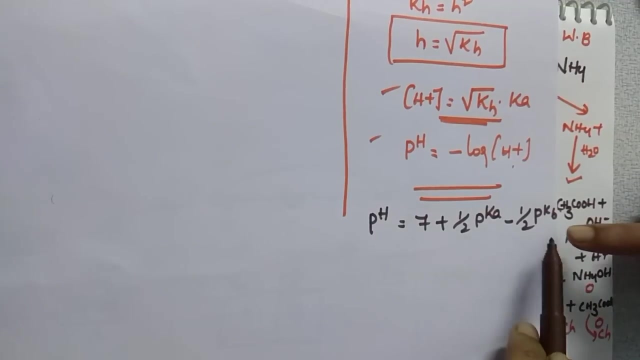 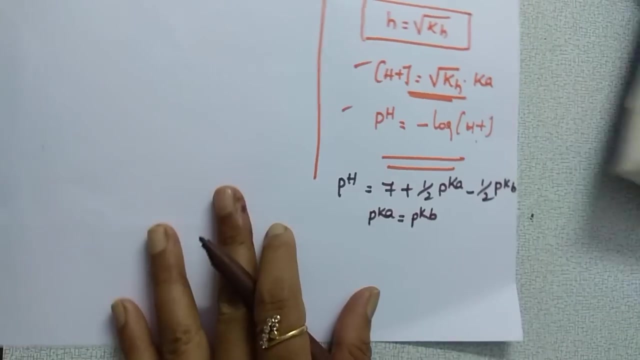 commonly, which is asking: See, this one is one more concept, Continuation of this, When This is a formula for calculation of pH for a salt of weak acid as well as a weak base. Suppose if pKa is equal to pKb, then what we get is pH is equal to 7.. 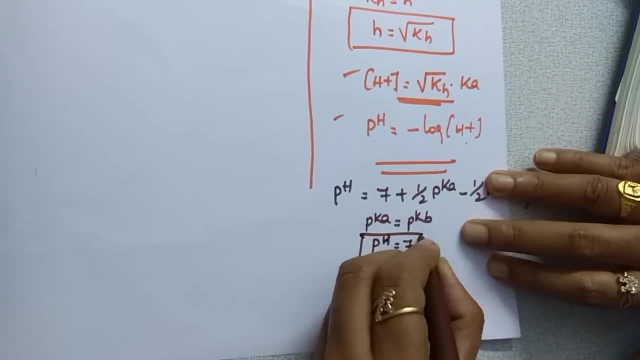 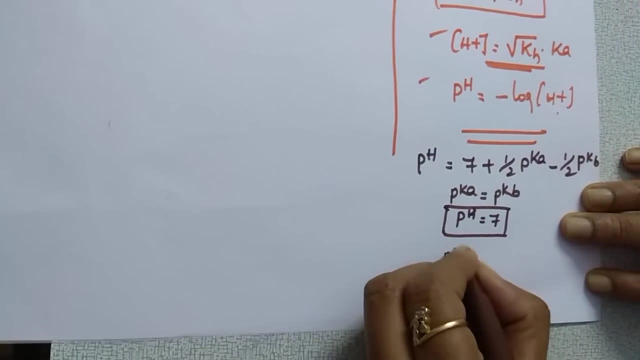 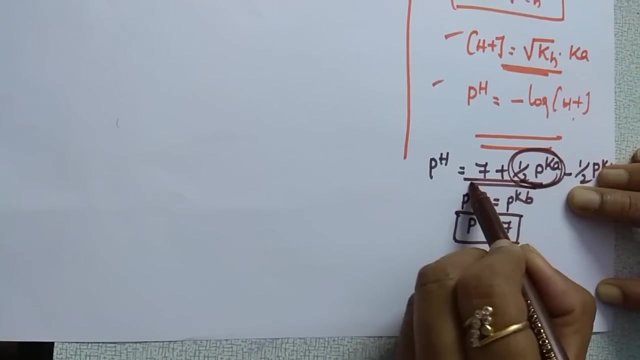 Clear students, pH will be 7.. Suppose if pKa is greater than pKb. then And suppose, if pKa is greater than pKb, which term is more? This term is more, So that positive term is more- then pH will be greater than 7.. 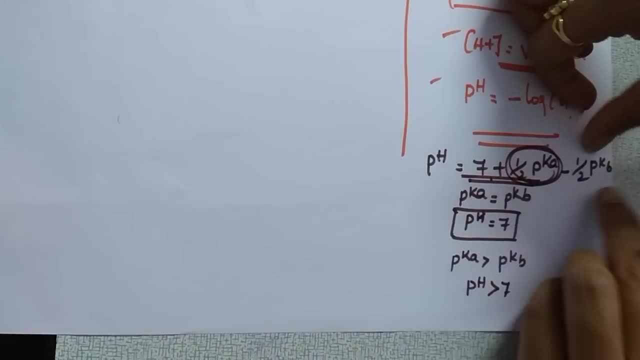 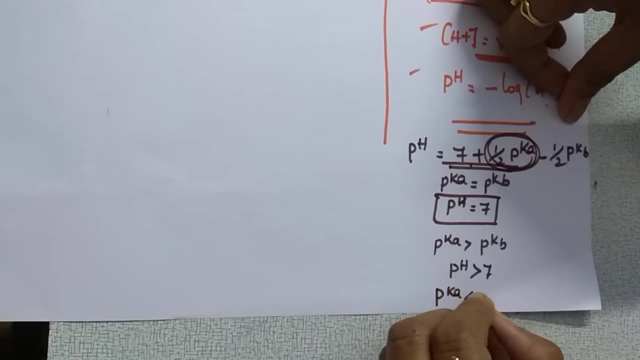 Clear, Easy students. If this term is more means minus, term is more, then that pH will be less than 7.. When pKa is less than pKb, which is more pKb is more, then pH will be less than 7.. 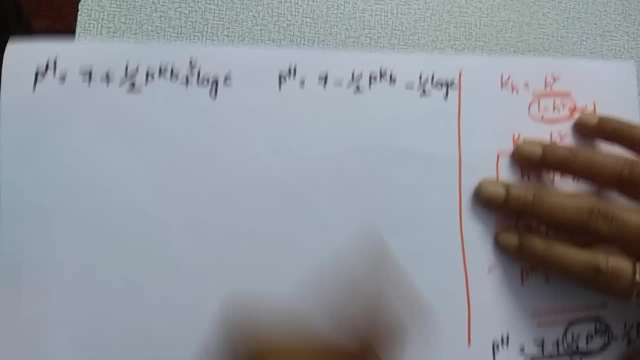 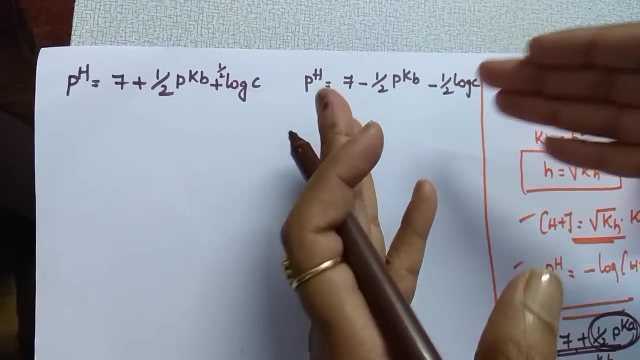 Just to prove Practice this. Don't listen and leave it Clear. And these two formulas will be given in your question and they ask you which is the formula to calculate pH for weak acid and strong base? Tell me Weak acid and strong base. 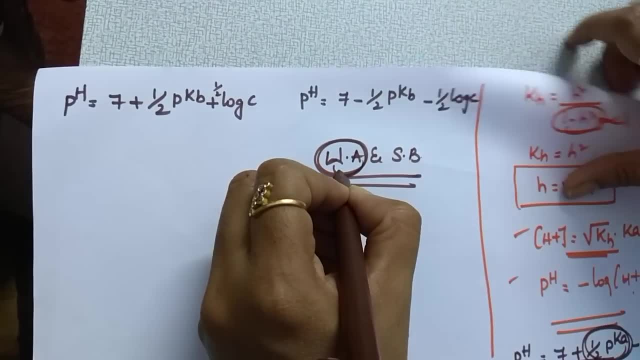 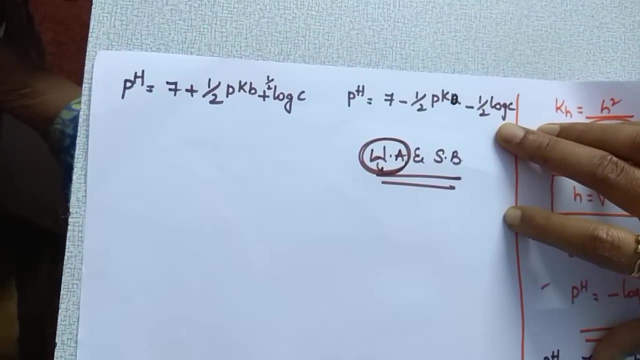 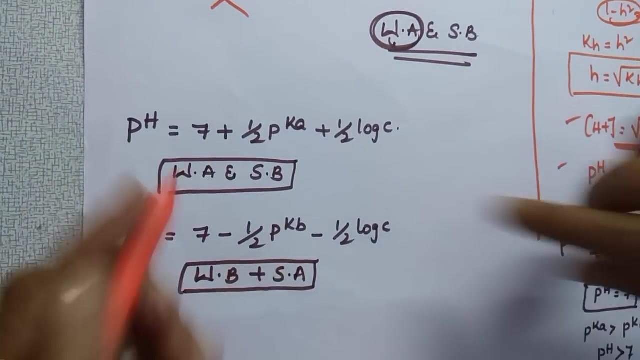 Clear. So whenever they ask weak acid, so that in the term it should have pKa, See here pKa, Not this formula, See this formula. Whenever they give you four options, just to see it, weak acid formula, always pKa will. 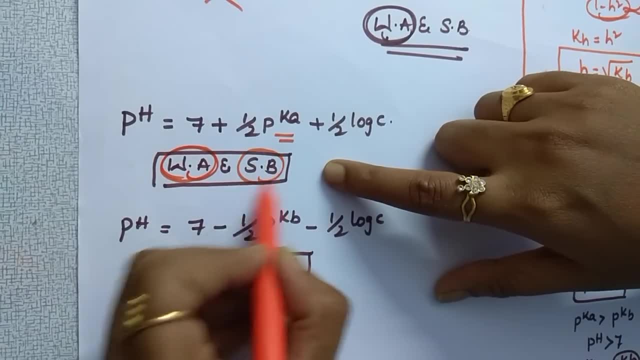 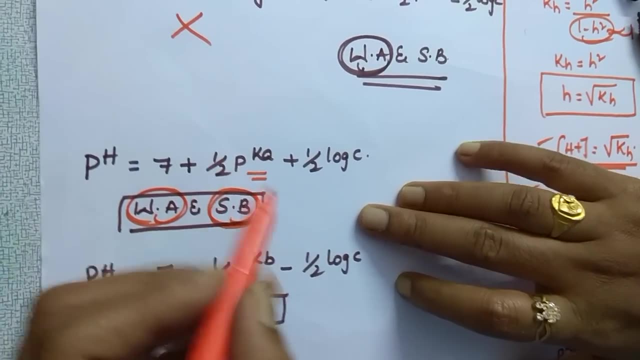 be there. Okay, And one more thing: Whenever it is a strong base, they are giving. no need to derive these relations in your exam. Not required, Just follow this trick: Strong base, Base, Always strong base means pH will be greater than 7.. 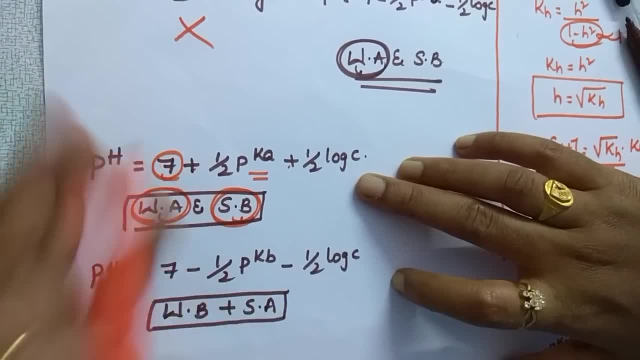 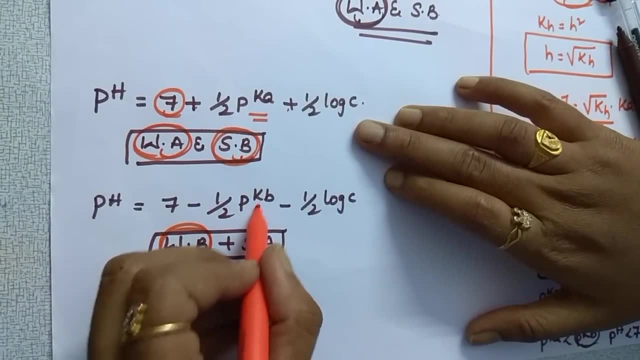 So all terms should be positive. Then only you will get pH greater than 7.. Next, Whenever they ask you for a salt of weak base and strong acid- Weak base means always pKa term should be there And they given that strong acid salt means for strong acid, always the pH will be less. 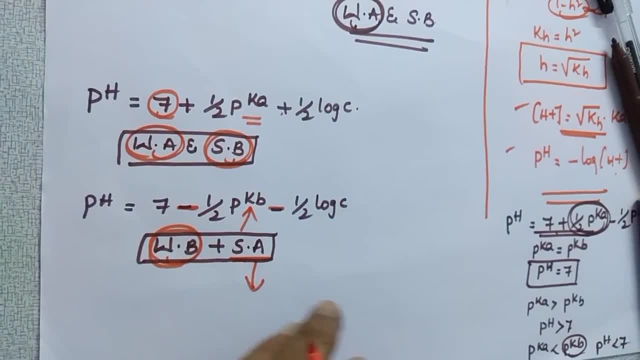 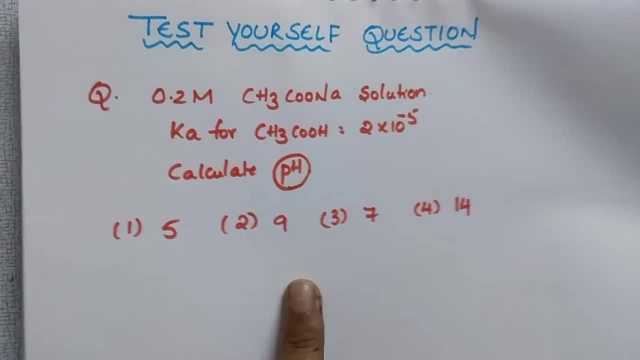 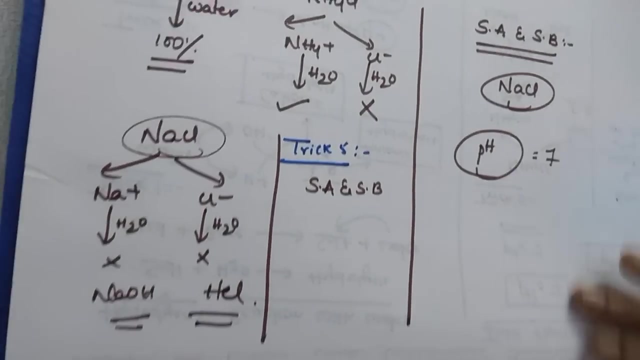 than 7.. So minus terms will be there. That's it, And go through this test yourself question. Solve this question and let me know your answer. And one more point I want to discuss: Whenever hydrolysis constraint H value, you will get this H. 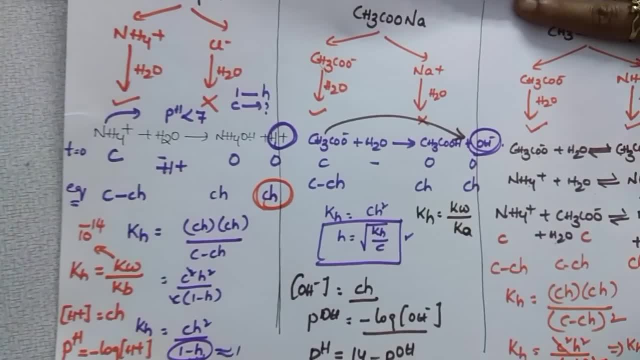 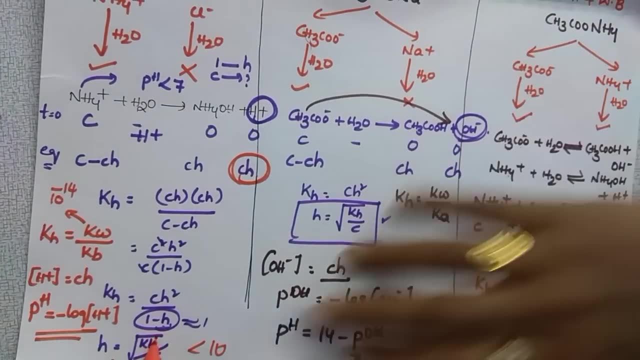 Whenever H value you get When you calculate H. Where is that Here? If you get this value less than 10 only you should neglect H value. Otherwise you have to use this only KH to calculate. Understand: H value less than 10%. 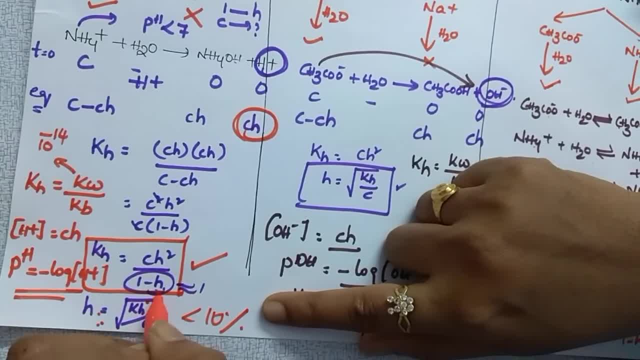 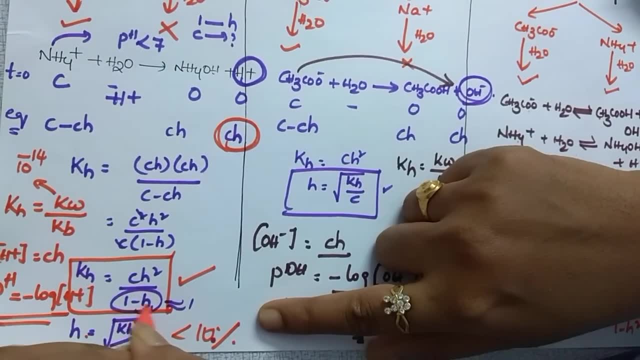 If you get, Then only you have to neglect here. This problem is correct. If H value you will get greater than 10%, Then you should not neglect here. 1 minus H. Direct formula you have to take and you have to solve by using quadratic equation. 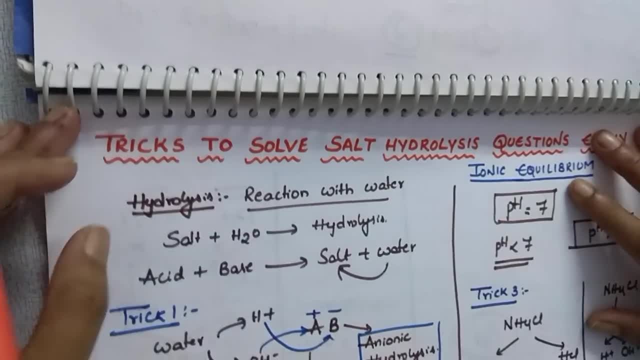 Thanks for watching. Please give like and till you didn't subscribe to my channel, subscribe it.